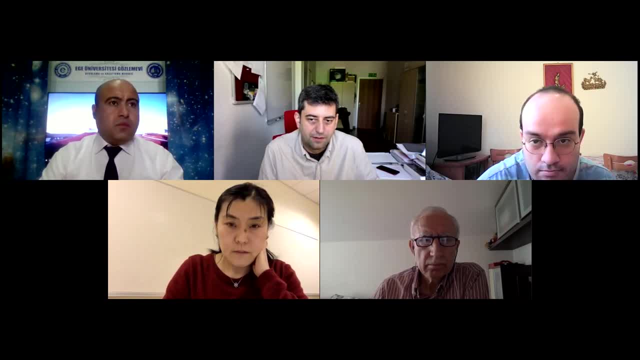 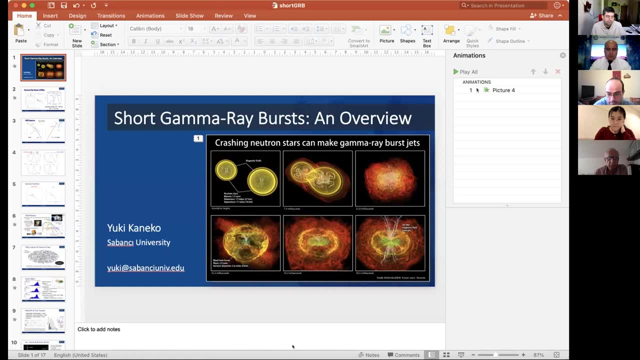 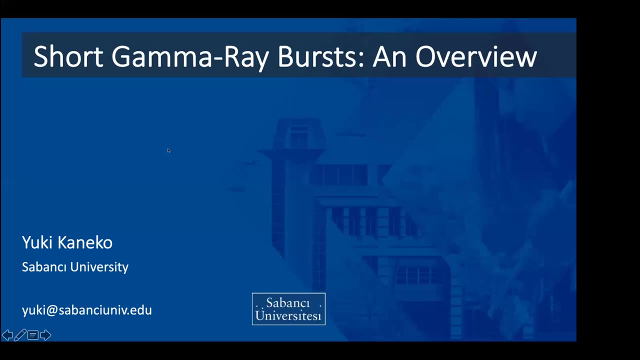 Okay, can you see the screen? Yeah, perfect, Thanks, All right, good, Hello everybody. I'm Yuki Kaneko and I will be talking about short gamma-ray bursts today, And thank you very much, first of all, for the organizer for this very nice workshop and inviting me to talk about. 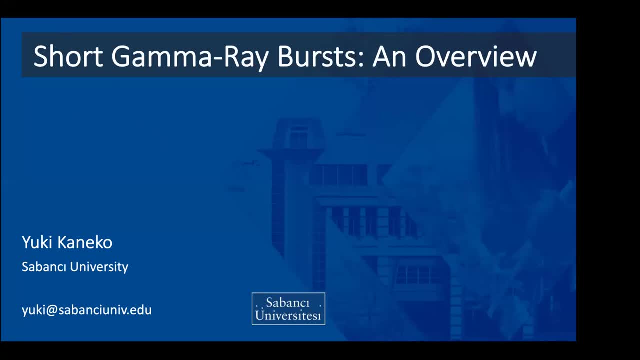 gamma-ray bursts. While I was preparing I noticed that you know talking about short gamma-ray bursts, giving overview in like 30, 40 minutes is very tough, So I decided to focus on the highlights- and you know main points of gamma-ray bursts and especially short gamma-ray. 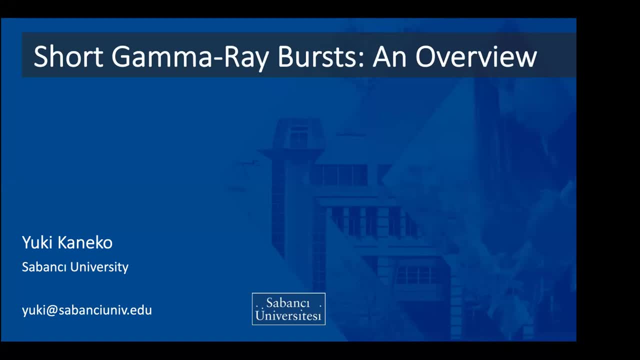 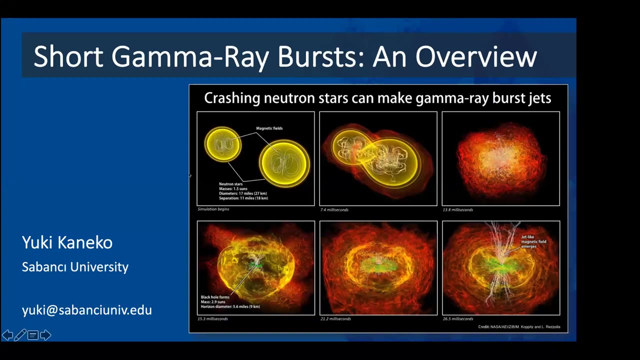 bursts. Some of you may be wondering. you know, if you're not familiar with short gamma-ray bursts, you know what's the connection between a neutron star and gamma-ray bursts. I'll try to make that connection. But later on today you will be listening about the merger of neutron stars and 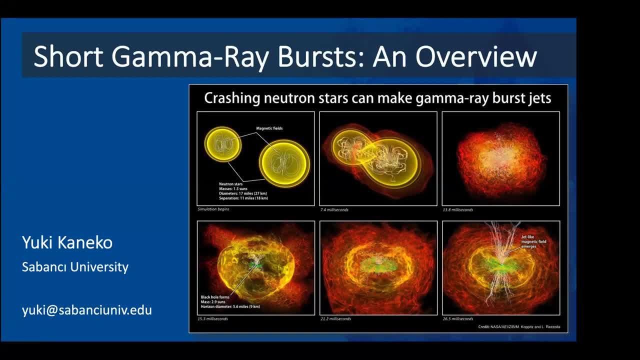 also CNM. I think after this we'll be talking about afterglow of gamma-ray bursts, So I will focus on observational points of view, observational facts from gamma-ray observation points of view. Okay, and so here is like a screenshot of a simulation, And this is a little, maybe, outdated. 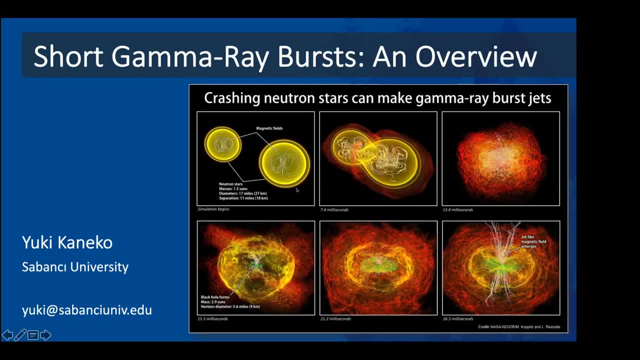 I'm not sure. I think this was a while back, But this shows how neutron stars may merge And then as it merges. this is a simulation of magnetic field lines and how it connects and then how this can launch some sort of jet. But I'd like to 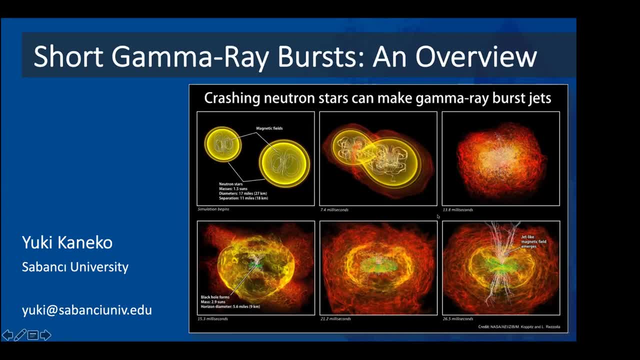 bring your attention to this millisecond timescale. It's, like you know, the whole thing is 26 milliseconds, So this happens pretty quickly. And then when the jets are formed, if we are in the right orientation, if you're, if you see inside of the jet, then that's what we see. 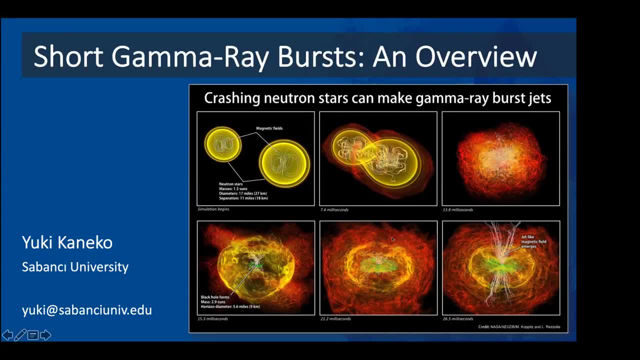 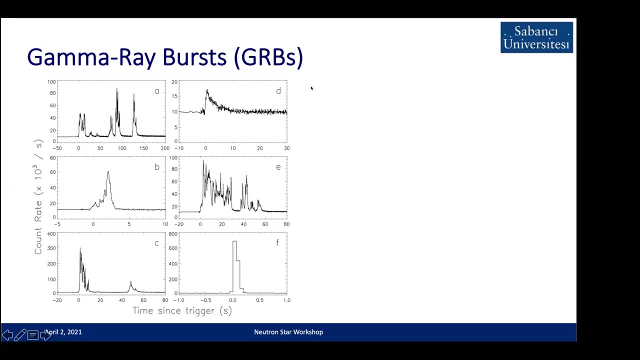 as gamma-ray bursts. That's what we think. So I like to connect to, you know, the observational point of view to this neutron star merger Gamma-ray bursts. you know it's very, very diverse, in a sense, in terms of light curve. 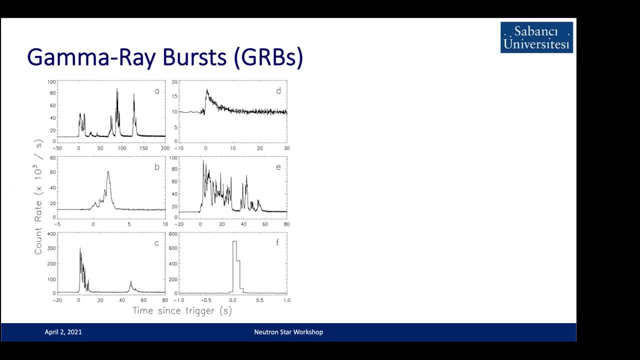 And then you can see the time in property, not timing, but how do you say the morphology as a function of time? So like these are one, two, three, four, five, six example of gamma-ray bursts And people used to say: you know, when you see a gamma-ray burst you saw a. 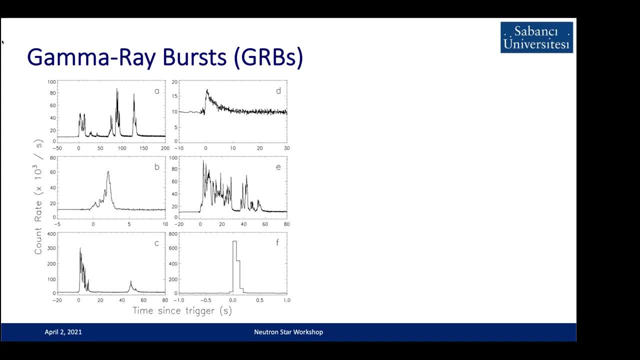 burst. you know it's so diverse that, okay, I saw, you know this one. it's lasting for 150 seconds, right, But then the next one is five seconds and it's only one peak or two peaks. 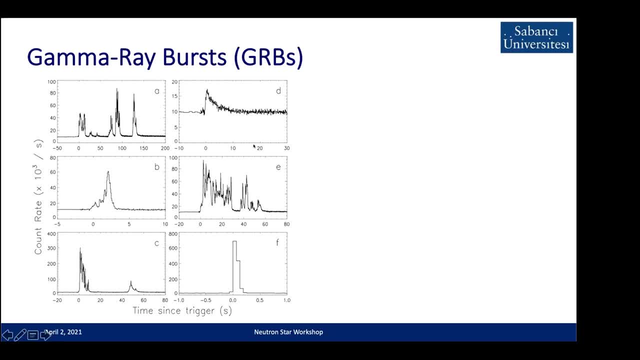 So here it's lasting for 60 seconds, 20 seconds, 60 seconds, And this is very, very short, You see, like this is one second right here. So this is in sub-second time scale, So we see all sorts of light curves And then, okay, but we can determine the duration of these. 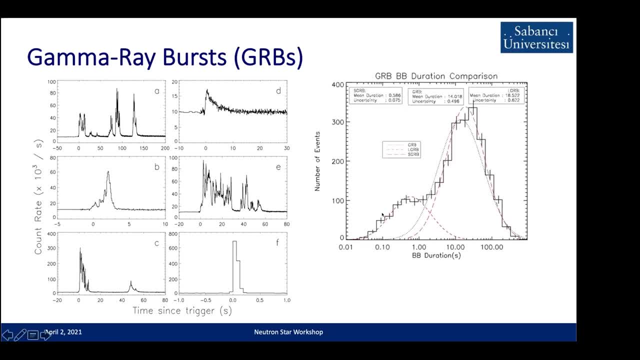 events And if you try to plot the duration or the population, the distribution of these durations, So this is a number of events versus duration of events, bursts, And you can kind of see a little bit of hump at the lower end And then there's kind of you know, this is in. 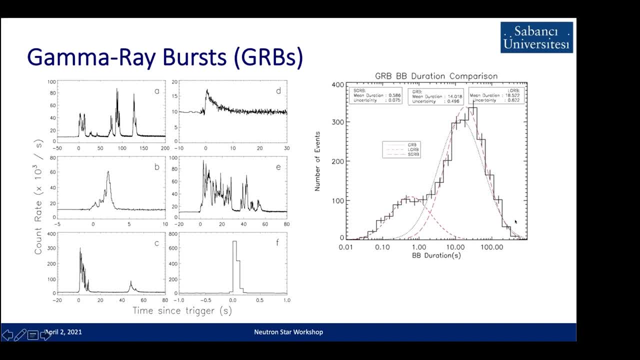 log scale, but kind of log normal distribution of this duration, And it goes in one, two, three, four orders of magnitude, four or five, even orders of magnitude in duration, in seconds And before. so this is actually the recent observation, observation of results from: 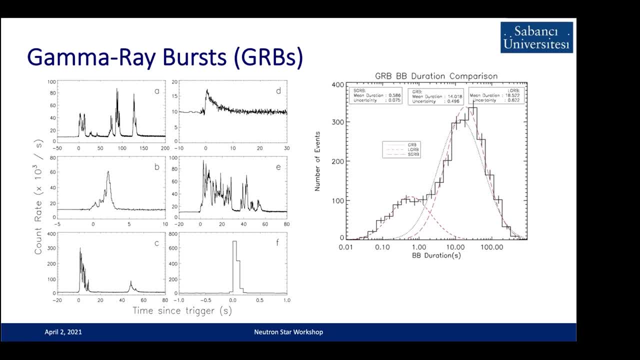 GBM. I'll talk a little bit about those instruments. But before this GBM, in 90s, we had another experiment called BATSI, and that's how you know. we know a lot about GRB to date And 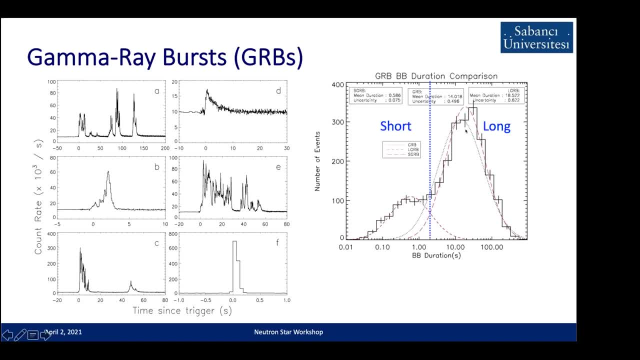 Based on that distribution, BATSE distribution- I will show it to you a little bit later- we kind of decided: okay, two seconds is, you know, a dividing line, that can you know, distinguish two different population of bursts, And that's historically, you know. just two seconds was picked but there's nothing clear as you can see, you know, from the distribution, there's not no cuts in a sense at two seconds. that divides, clearly, divides short and long events. 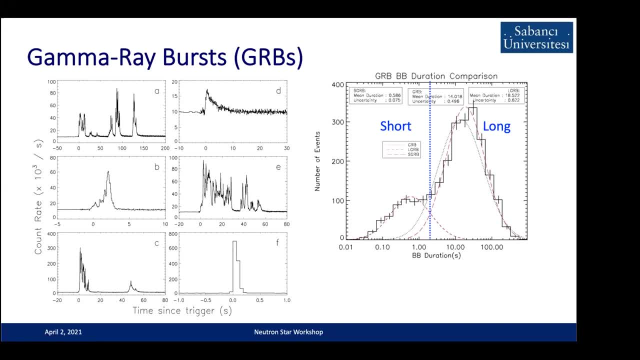 So when we talk about short GRBs, yes, we are talking about these events, GRBs that are- the duration is shorter than a few seconds usually, But it could be like up to five seconds or so because the distribution for the lower one it goes. you know, there's quite a number of events that could belong to both short and long. 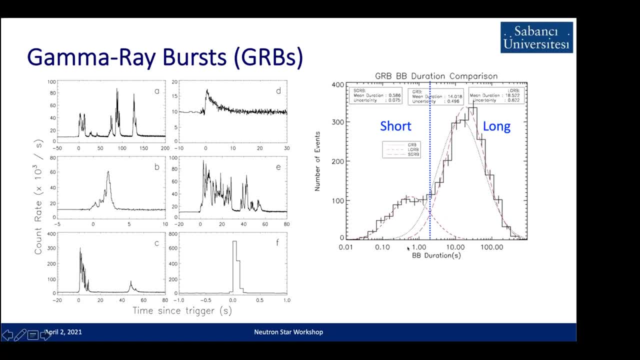 Okay, so this is kind of dividing line And in general, when you estimate how much energy is emitted in gamma rays, in these you know both short and long. the total energy is about 10 to 51 to 2.. 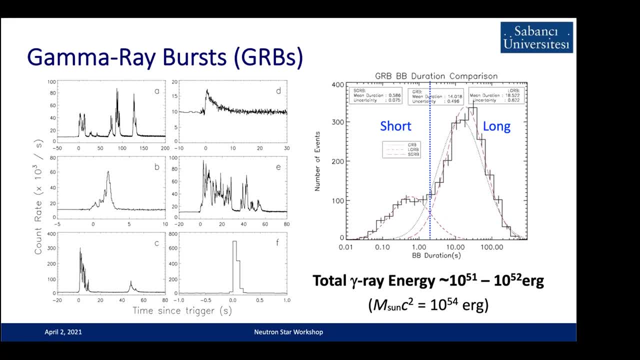 And that, you know, is of the order of rest mass energy of the sun. So imagine the rest of mass rest mass energy of the sun is released in, like you know, 10 seconds or even like one second. So that's a lot of energy and a lot of energy released that we're talking about. 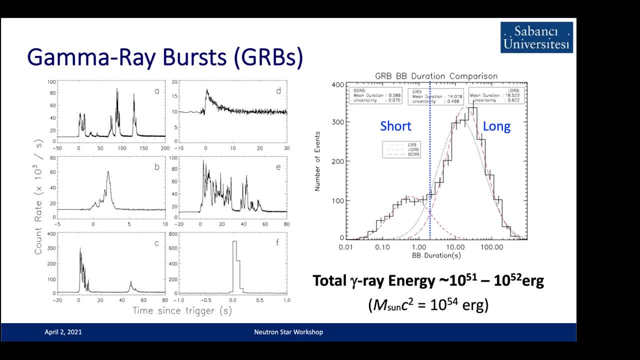 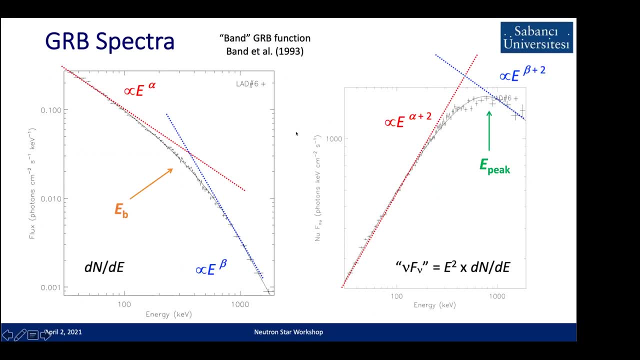 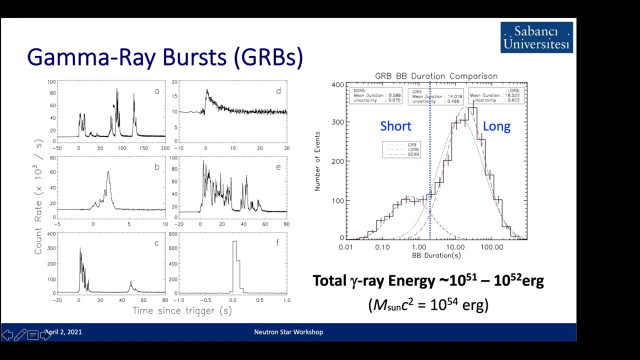 So we need to have some sort of a very, you know, catastrophic event, a very strong event that produces this. Okay, But on the contrary, if you look at the GRB spectrum, energy spectrum- it's actually pretty constant. So it doesn't matter you know which one, but you know chances are any parts of these events, this one or this one, or it doesn't matter. 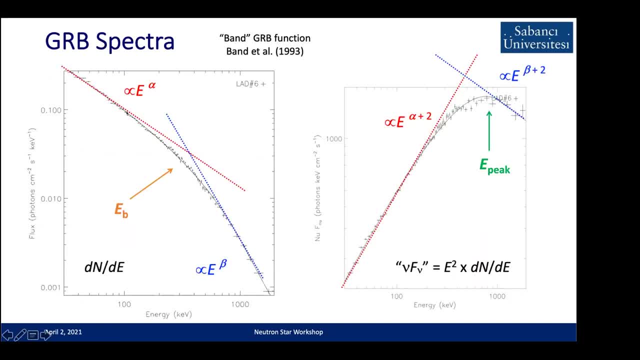 You can describe the spectrum in this. what's called the bands function was proposed by bands in 1993.. And we still use this function to describe the spectrum spectra of GRBs. And this is what this is is actually just the two power loads connected with each other. 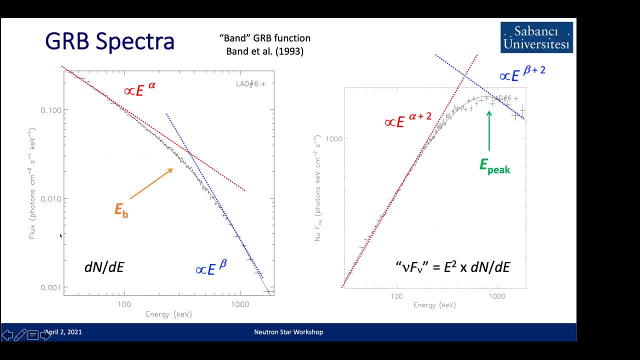 So this is an energy spectrum. It's a photon counts, the photon flux actually as a function of energy. And these are. these are both log scales, So you have the power load function as a straight line here And you have a low energy function. 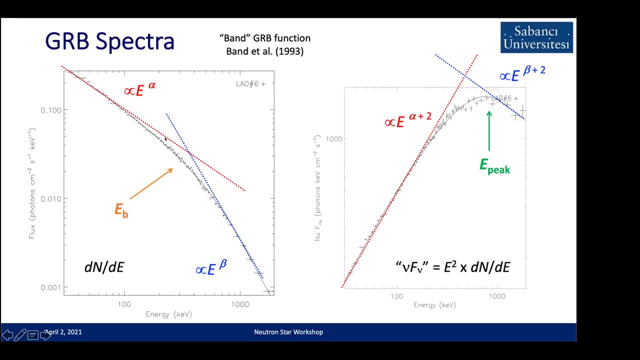 And you have a low energy power and high energy power connected kind of smoothly at some break energy. But when we talk about energetics or the GRB spectra parameters we use a lot this terminology parameter E peak, And this E peak is a little bit different from E break. 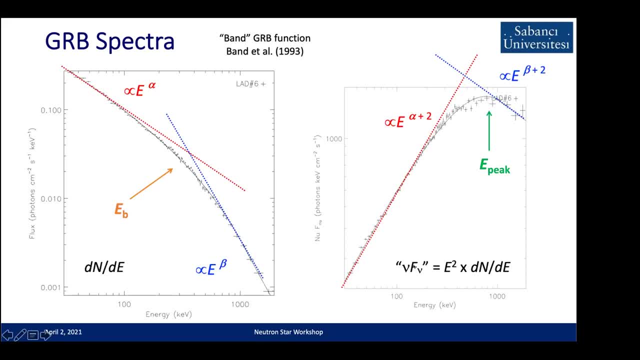 But this is the peak of what we call new F, new spectrum. And for those of you who are not familiar with spectrum, New F, new is photon flux per energy is here And you just integrate that twice over all the energy. So it's, like you know, E squared times this photon flux. 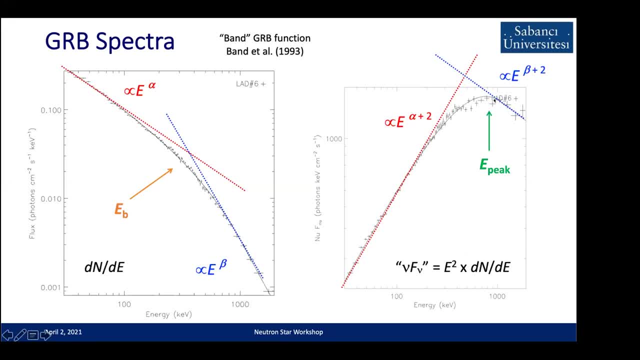 And this becomes the new F new which shows how much energy is emitted at which energy band. So here E peak is around one MBV, or a little bit less than one MBV here. So the most of the energy, or the most energy, is emitted around this energy band. is what it means. 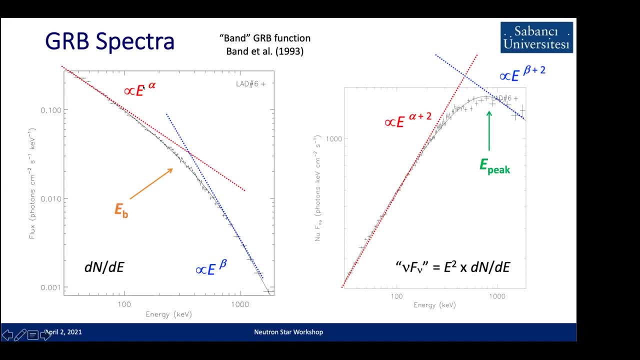 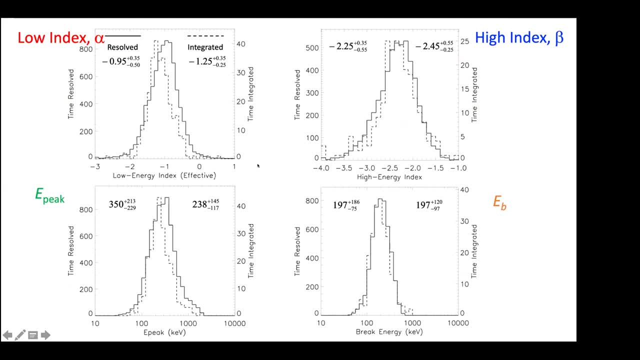 So then, if you look at the distribution of this alpha, beta and then E peak, The distribution is pretty narrow, I will say, you know, for the diversity of the light curve that we observe. So this is like a distribution of time resolved spectrum. 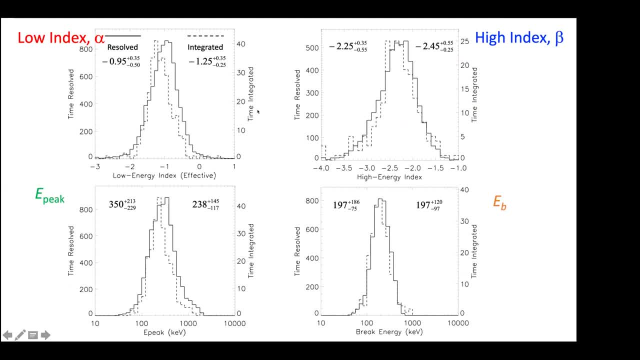 And also the time integrated spectrum, The whole burst or the you know, each time bin spectrum. But you can see that in both cases alpha is around minus one, Beta is about minus 0.2.. E peak is about 200, 300-ish here. 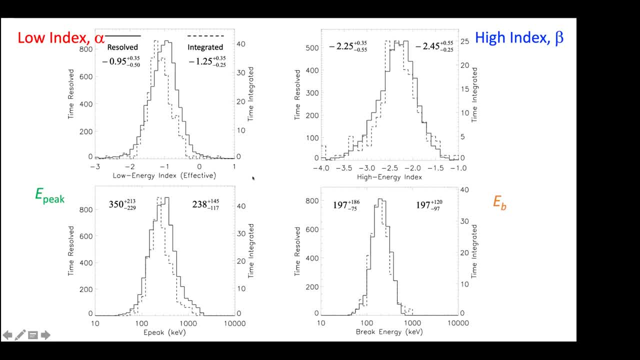 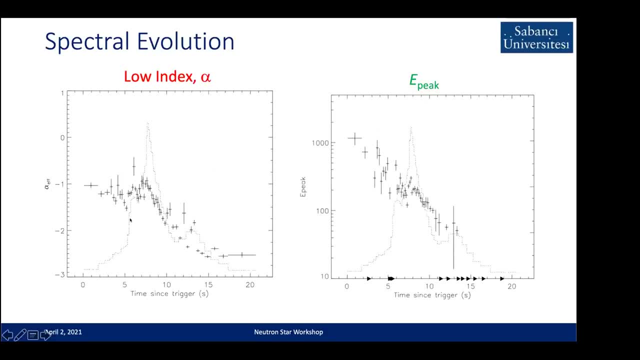 Okay, And this time integrated and resolved spectrum. And this time integrated and resolved. it matters because within the burst- Like this is one burst. just an example: You can see the light curve in dotted line in both cases And this is as a function of time. 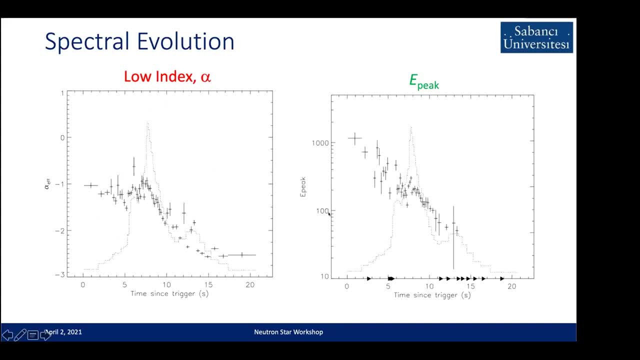 This is alpha, the low index, And this is E peak. And you can see that both alpha and E peak varies a lot during within a burst Right. And this kind of evolution we call it hard to soft because it does, you know, go from hard E peak to low E peak. 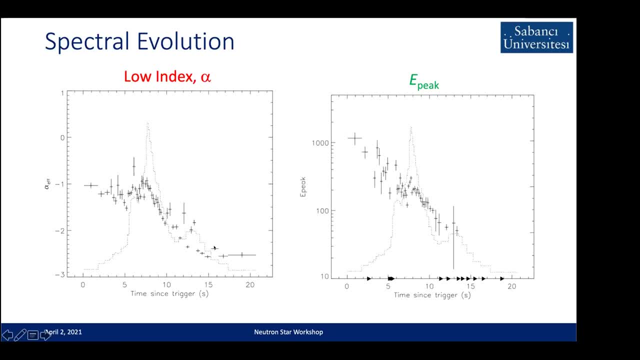 And also the alpha becomes fairly, you know, soft as it goes, as the time goes, And this is just one type of evolution that we see. We do see other events that have that tracking behavior. So the hardness of the spectrum actually tracks the photon flux. 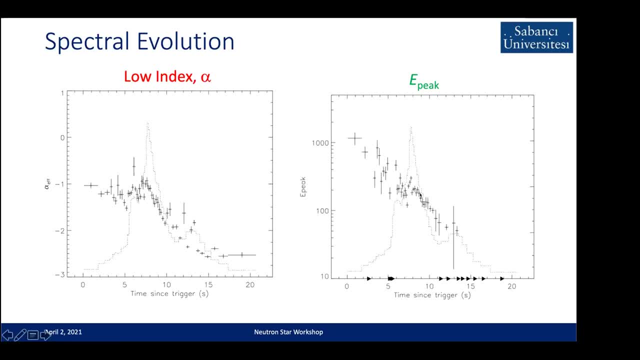 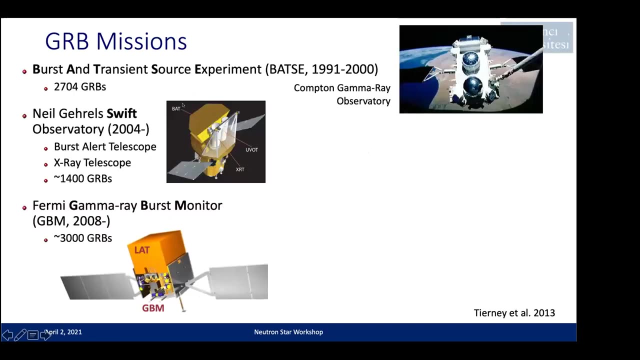 So the brightest part is the hardest And the dimmer one is dimmer part is softer. Okay, So spectral evolution was their variety. And who observes this? Or we observe it, but we observe with which instrument Right? So in 90s, as I mentioned, burst and transient source, experiment BATI was you know. 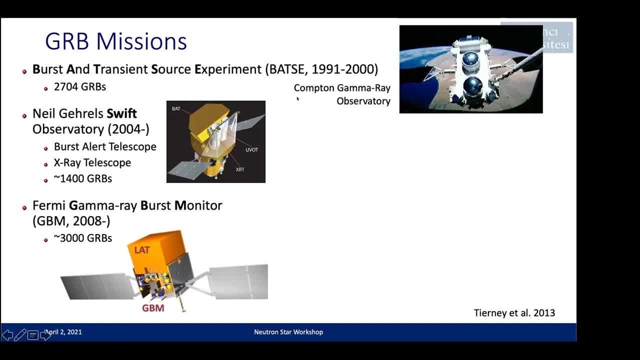 specifically designed to detect GRBs And it was on top of Compton Gamma Ray Observatory. This was very special. actually, This is an actual, real picture of Compton Gamma Ray Observatory taken by astronaut in space shuttle, And it's pretty cool because this was really heavy. 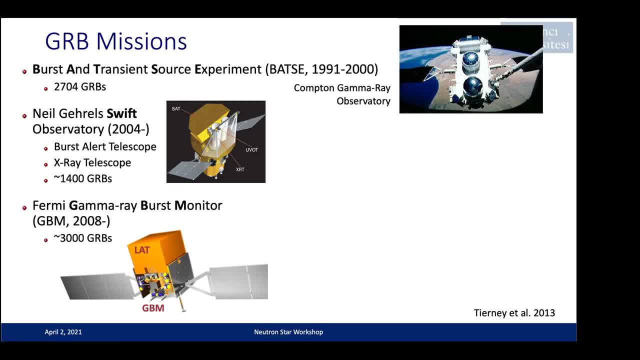 It was a huge observatory that it couldn't be launched with a rocket, So it had to be launched with the- what is it? A space shuttle, Okay, So this is one of the coolest pictures that I have, And it observed, in nine years, 2,700 GRBs. 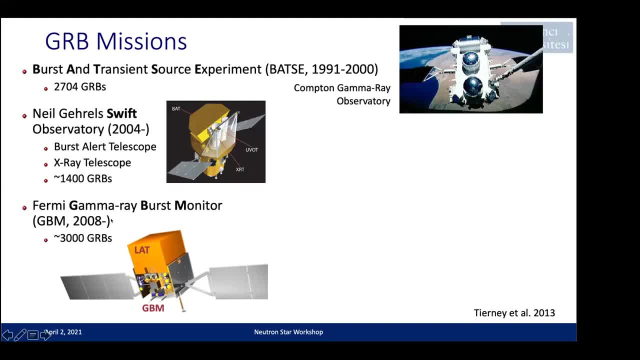 And right now we have Swift and Fermi telescope in orbit And they're actively monitoring, observing GRBs. right now And so far the Swift Burst Alert Telescope is right here- Observed about 1,400 GRBs, And then Fermi Gamma Ray Burst Monitor, GBM, have observed about 3,000 GRBs. 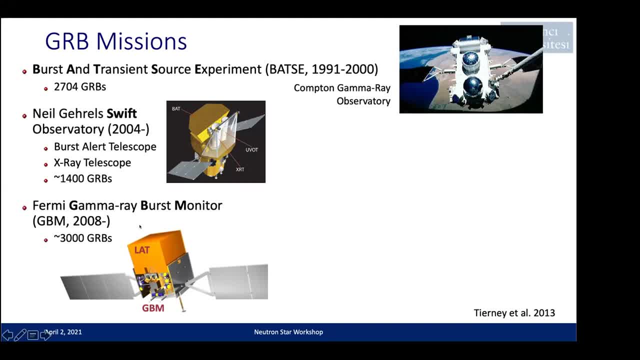 So we have observed a lot of GRBs, So we have, you know, a lot of data to work with. But also the short GRBs are not, you know that many compared to the long GRBs? Okay, And these all these are sensitive to this: 100k BATI. 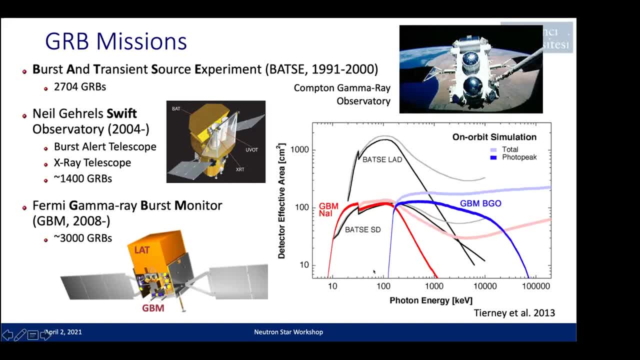 100k BATI to one may be like this area, this energy range. So this shows the effective area. So this is kind of the sensitivity of the detectors And for BATI, for two different detectors of BATI, that is the black curve. 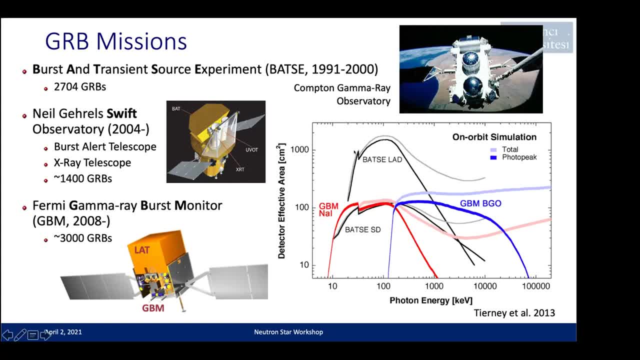 And it shows, you know it's sensitive about around 100k BATI. And then here red and blue are GBM detectors. So GBM has two different type of detectors, But you can see that the coverage is a little bit wider now the energy coverage. 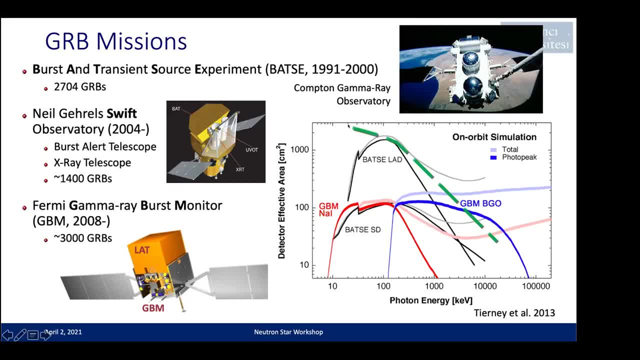 Okay, Compared to BATI And the earlier spectral shape that I showed, you know kind of falls in here. This is about 200, 300k BATI here. So this is there's energy break right here And then it goes something like this: 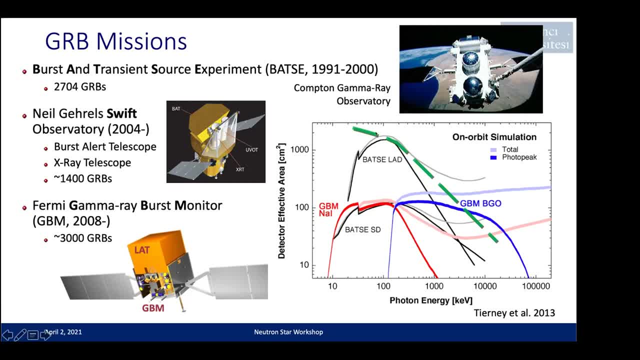 Okay, So these are all designed to be most sensitive around this break energy, Okay. And then, lastly, the BATI- Swift BATI sensitivity goes something like this, And Swift BATI has a great capability of localizing the events really really well. 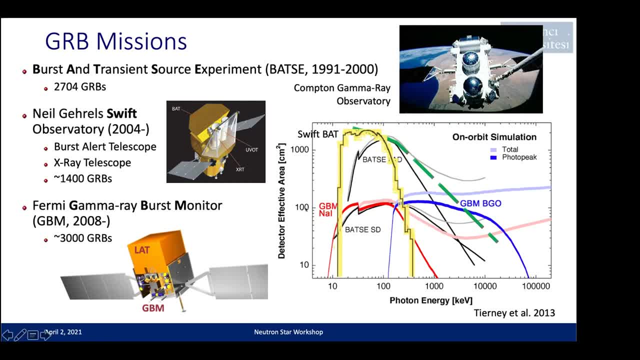 BATI and GBM does not have the localization capability because it's all sky monitor And I'll show you why it's all sky monitor in a minute. But Swift BATI, if it's observed, if the GRB is observed with the Swift BATI, then most likely it can be localized. really nice. 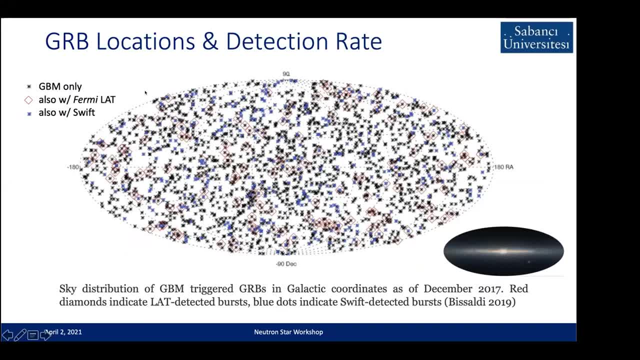 Well, okay, And location of GRBs. you know it happens in all over the place. So this is a galactic coordinate location plot of all GRBs that we have has been observed with GBM, Okay, And you may have seen a galactic coordinate picture of this galactic plane. 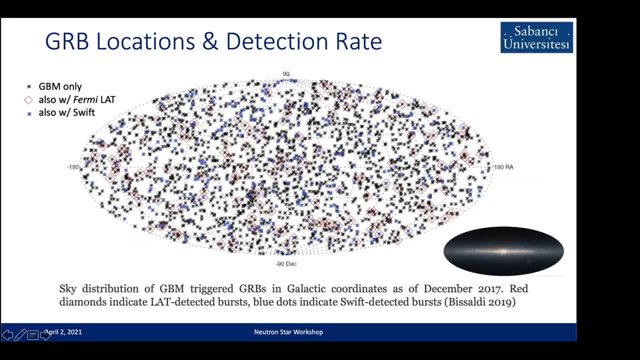 So if it happens in galactic plane it will be along this horizontal line, at the center, like this. So, as you can see, it really happens all over the sky And because of that, BATI and GBM, both are made to observe all sky, to kind of monitor, you know, try to catch as many GRBs as possible. 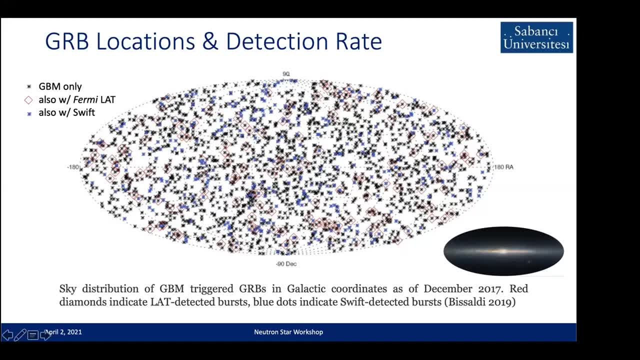 Okay, And some of them you see, like many blue points here. I don't know if it's visible to you, but these are the ones that are observed with GBM and also with Swift BATI, So there are quite a number of them that we have, both detectors or observatory observing these events. 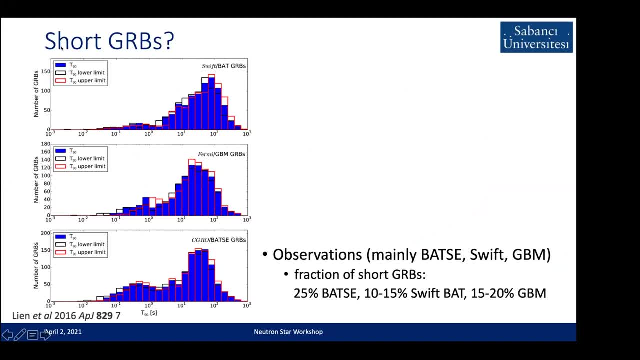 Okay, And short events, Okay. Okay. I showed you a little bit earlier the Fermi GRB duration distribution, But here's a comparison. BAT GRB duration distribution is like this: This is Fermi GBM. This is BATI. 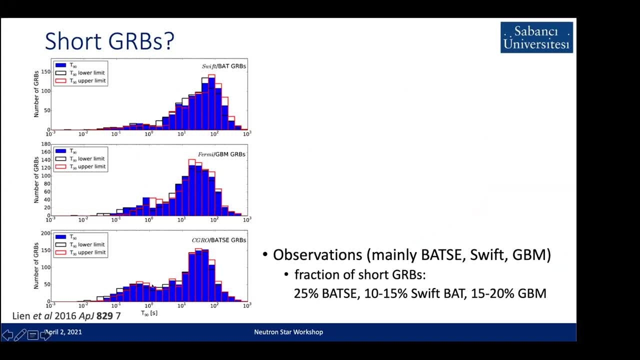 And you can see that the BATI distribution shows a little more distinctive kind of value here right around two seconds, And that's exactly why we chose two seconds. As you know, not we but people usually choose around two seconds historically. 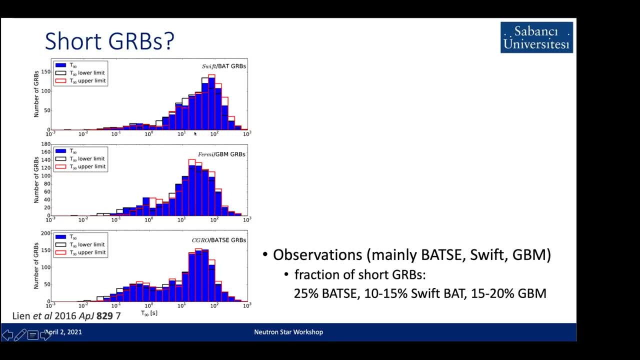 Okay. But after BATI, when we start observing GRBs with BAT and GBM, we saw that this distinction is a little bit less, So it seems like more. you know continuous distribution: Okay, So there's still. you know a lot of people started trying to study the classification of, you know, short population and long population. 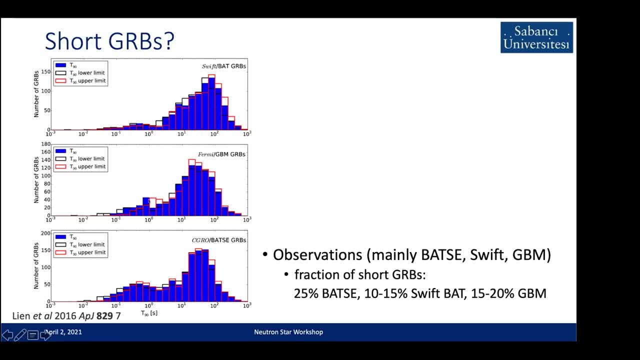 Okay, But it seems like there are two populations, but not that clear And you can see from these plots too: BATI observed the most, the highest fraction of short GRBs, It was about 25% of all BATI events were short, less than two seconds. 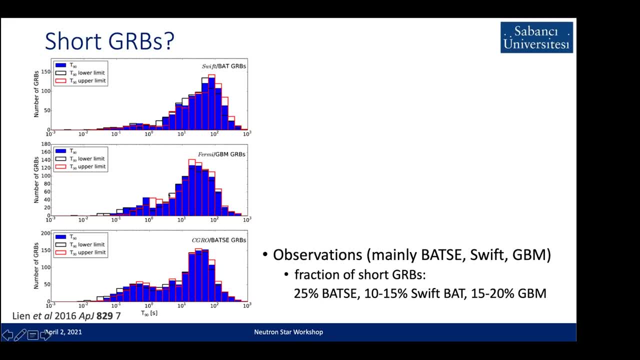 And SWIFT-BAT and GBM is much less. It's detecting much less. You know it could be dependent on The sensitivity detector, sensitivity or trigger mechanism, But for whatever the reason, it's really detecting a little bit less. 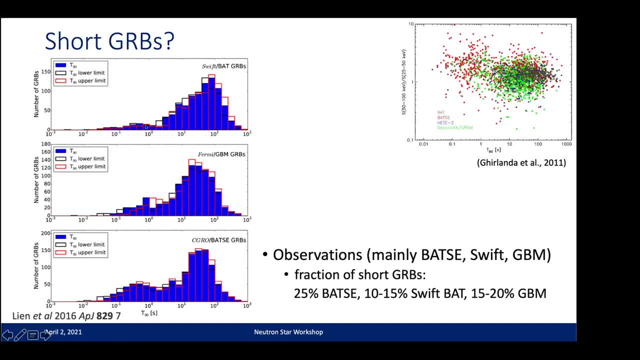 And other things that distinguishes short GRBs from long ones, is the hardness Not exactly distinguishing. actually, I must say You can see here the hardness ratio, the flux of hard energy and low energy Versus T, Versus T90.. 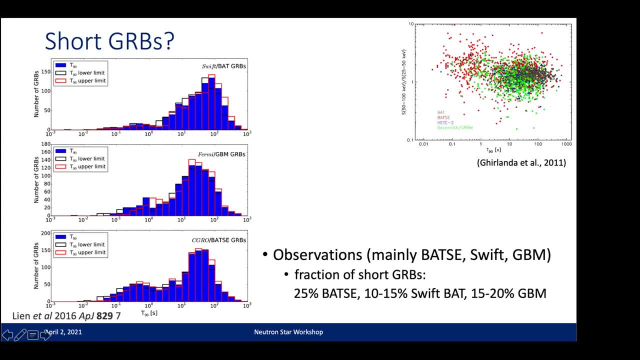 So two seconds is around here. Right, You can say there's a tendency of short events being a little harder spectrally, But you know you don't see a really clear correlation here either. Okay, But for other, you know, whatever the instruments that we see when we plot hardness versus duration, this is what we see. 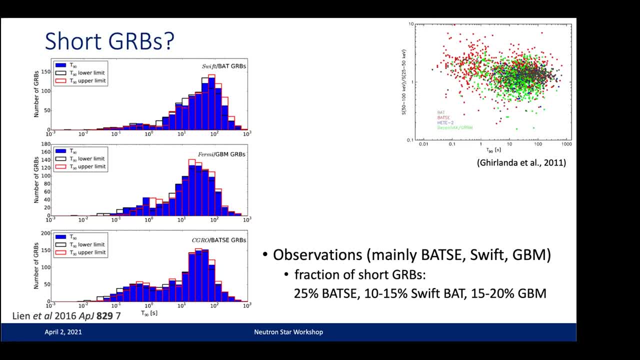 The shorter ones tend to be a little bit harder, And that's why some people call it short hard GRBs and long soft GRBs, And this is why. So, in addition to spectral hardness, there are some differences, But again, because the sample sizes are much smaller in short GRBs than long GRBs, we have less information to work with. 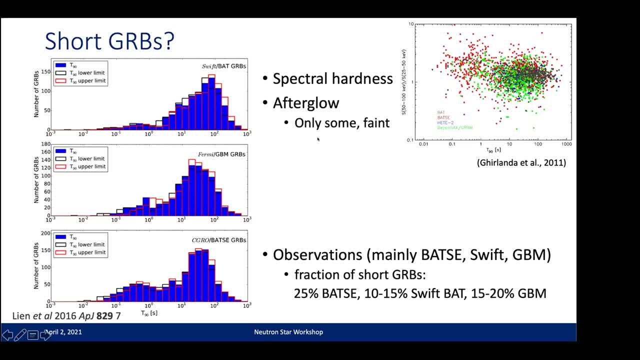 But we do have some afterglow observation of these GRBs. Afterglow is what happens to electromagnetic radiation at lower energies- X-ray, optical and ultraviolet optical radio. that is observed right after the gamma ray burst And because short events are very short and it's really hard to localize right away. 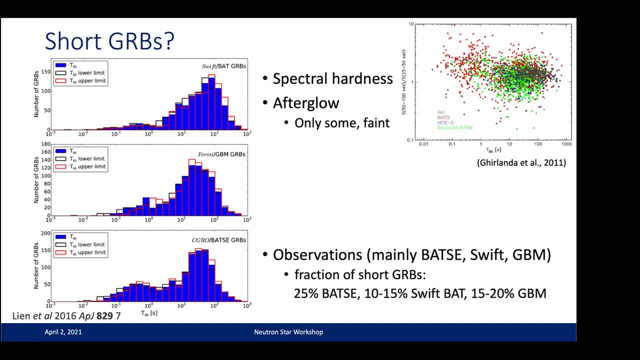 And then try to catch the afterglow light. But we do have some observations, especially in X-rays. We have, you know, probably almost close to 100, maybe because of SWIFT, But we have very few radio observation, for example from short GRBs. 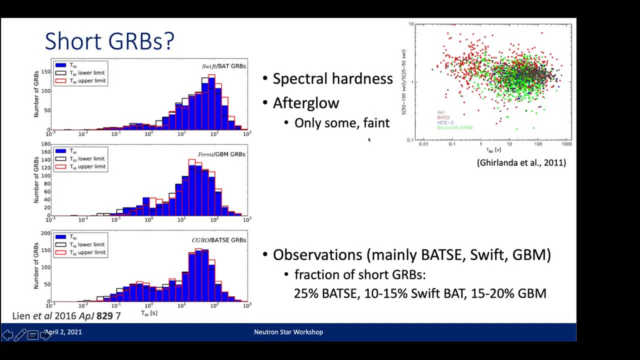 And they're thought to be happening in a very faint- The afterglow is thought to be expected to be faint- actually because of the X-ray. So in the environment that neutron star merger happens. I'll mention it to you a little bit later. 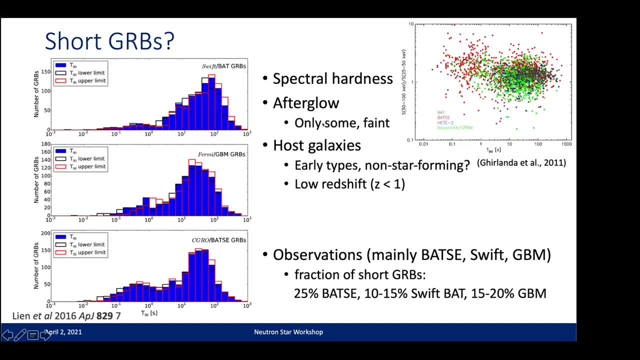 Okay, And also for those who Those events that we were able to localize based on afterglow observation and determine the distance or the host galaxy based on optical observation, We can see that there are mixed types actually of host galaxies. 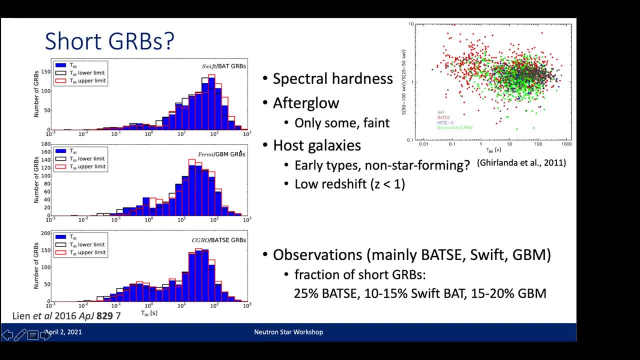 Long GRBs. many of the long GRBs, most of the long GRBs with afterglow host galaxies, are identified to be star-forming galaxies. But for short GRBs we can see that some of the host galaxies are early type, some are late type. 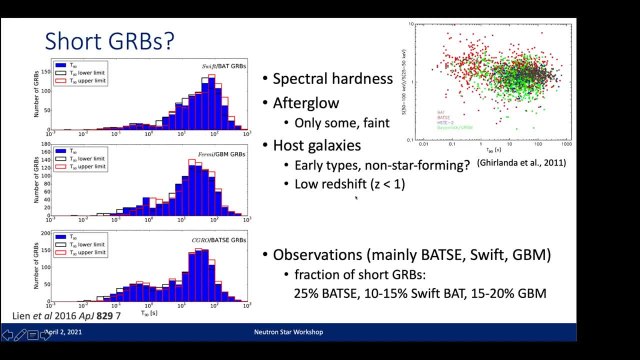 So you know they're still not really settled The case here, But all, almost all GRBs- short GRBs- that we have been able to measure redshift, of cosmological redshift we were talking about. So that tells about the distance. 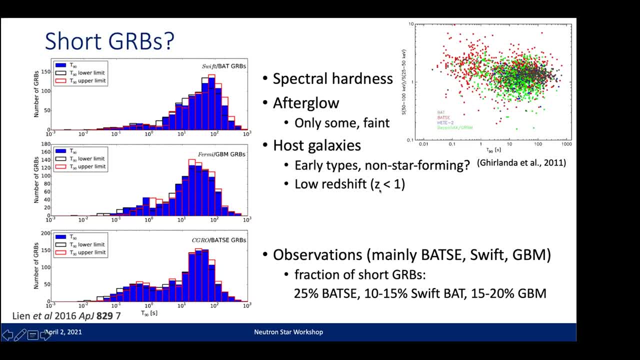 They're all low redshift, less than one. So you know what we're detecting is very close by. actually I'll show you this little bit More information in the next slide. And the progenitors you know the most, the strongest candidates is a neutron star or compact object merger. 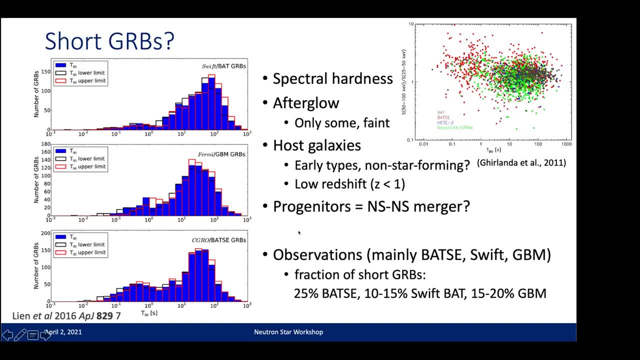 And I'll show you some evidences that we have for that. And then we have some extended demission- short GRBs with extended demission. That really complicates the things you know issues even more. So I'll try to mention all of this for the rest of the talk. 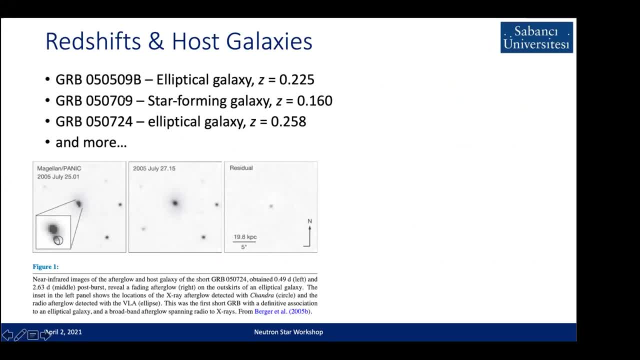 Then afterglow, of short GRBs It's. we have quite a number of X-ray afterglow observation because of the SWIFT, as I said, But optical observation is needed for determining the host galaxy And then also, you know, getting the spectral lines for the cosmological redshift, to determine the redshift value and determine the distance. 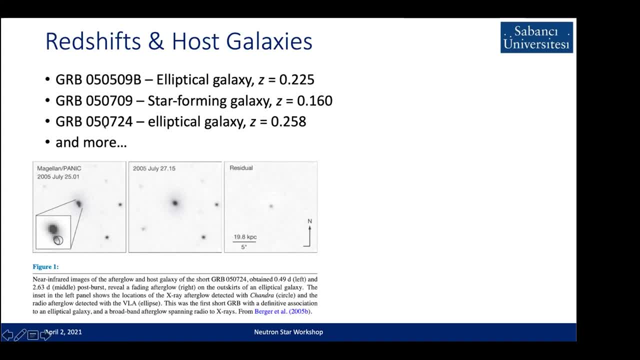 So in 2005, there are these three events that came out like on top of each other almost with all, with the afterglow observation, And this one in May was observed to be an elliptical galaxy And then the next one in July turned out to be was in a star-forming galaxy. 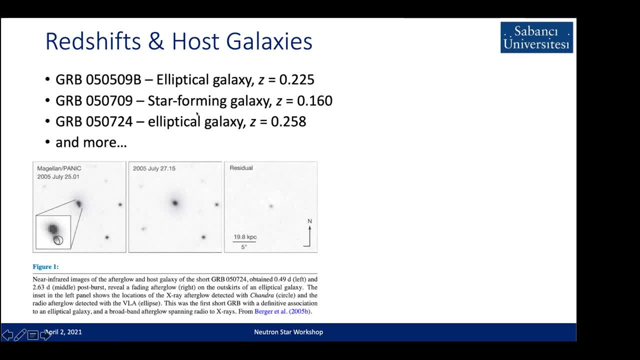 And then the community was really puzzled, Guess which one. And then the third one in July, later July, there was one more observed in elliptical galaxies. And then this one is for this: 050724.. This is the actual optical observation of this event. 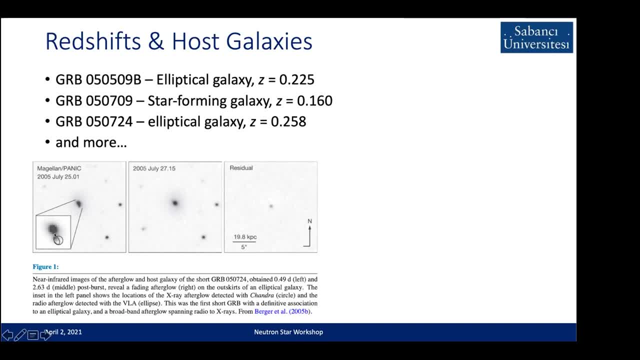 And you can see the elliptical galaxy, And then you can actually locate the GRB. This is the afterglow of GRB in optical And this what's happening in outskirts of the galaxy, the host galaxy, And this one also in a star-forming galaxy. 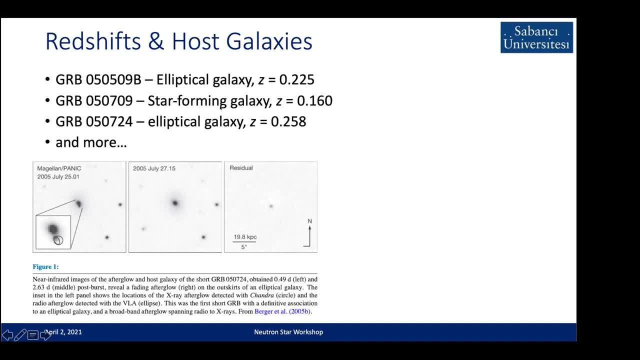 But this one also was observed at the outskirts of the galaxy. So that is actually consistent with a neutron star merger scenario, because you know those could be happening. Those should be happening in an elliptical galaxy, Those should be happening in an early-type galaxy because the star has to have evolved to those merging ages. 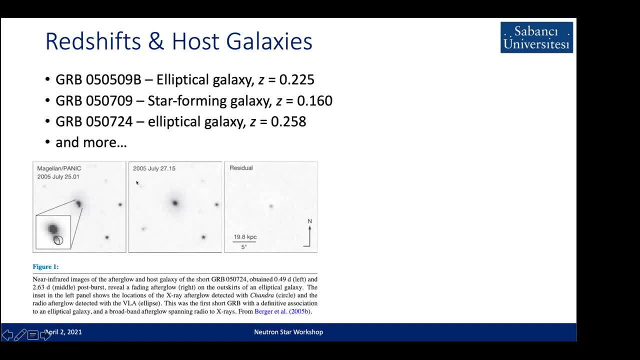 But because when they merge and when they form black hole or magnet or whatever you know the even more compact object, there has to be some sort of kick velocity And that will just, you know, kick everything to the whole system, to outskirts. 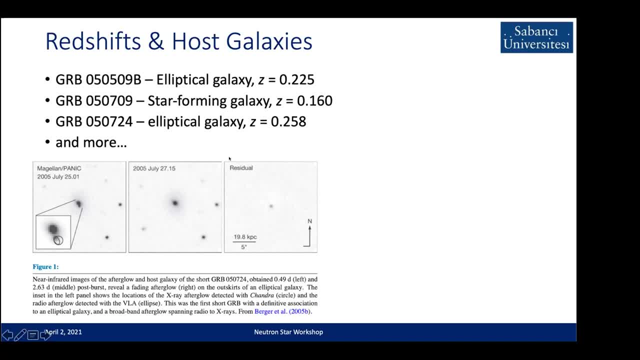 The whole system to outskirts of the galaxy anyway, And that's why the afterglow is expected to be dimmer. yeah, the less bright- Because afterglow is, it depends on the interstellar medium density. So outskirts of the galaxy, of course density is lower there. 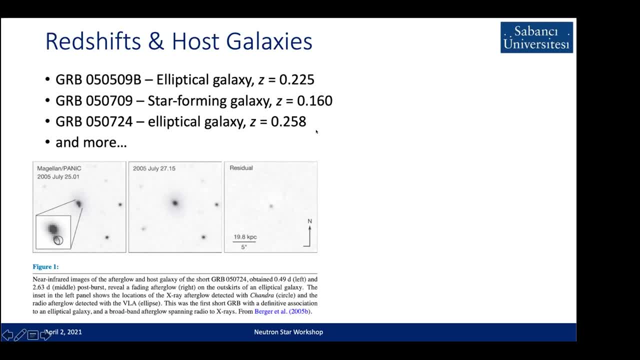 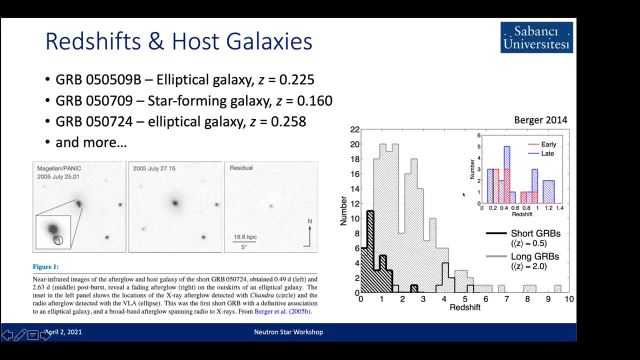 So that is, you know, still consistent. But we do have many more observations of host galaxy, of what is it? short GRBs, Yes, But it's still not settled. You see, here this is from Berger review of short GRBs. 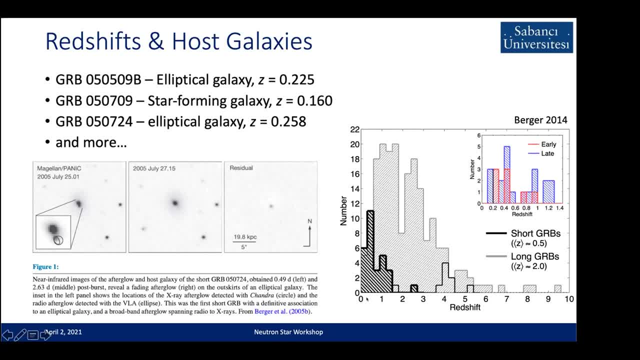 So this is a number of events- short- yeah, all short and long events as a function of redshift. Okay, The long GRB redshift can go pretty high. This is still kind of debated. I think It's not confirmed yet. 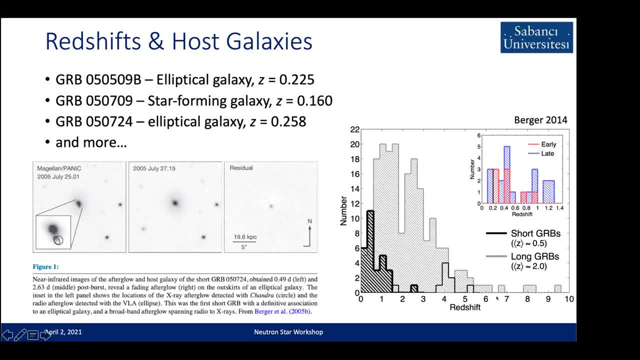 But you know, eight redshift is pretty. we have like a few of them there. But anyway, if you look at the short GRB redshift you can see that. so we do have something more than one. Yeah, I correct what I said. 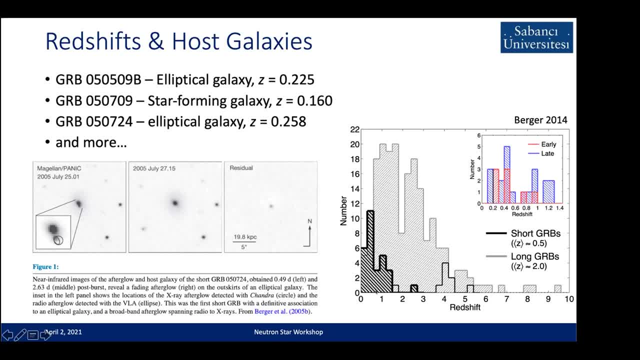 But on average, you know, most of them are less than one in redshift. Okay, So all the most of the short GRBs that we observe happens close by. It's not that it happens close by, but we observe that the ones that's happening close by. 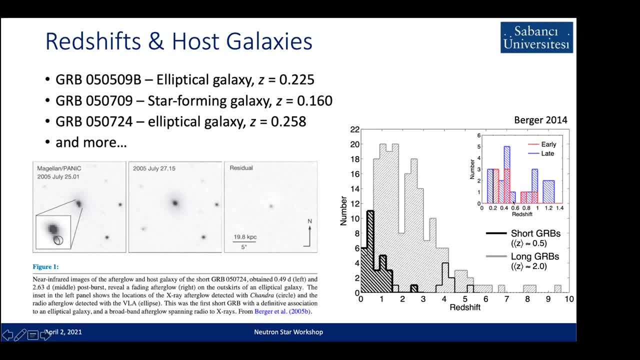 And then this is the type of galaxies: host galaxies for short events. You can see that it's, you know, some of them are late, some of them are early. So you know, the type of host galaxies can vary, Okay. 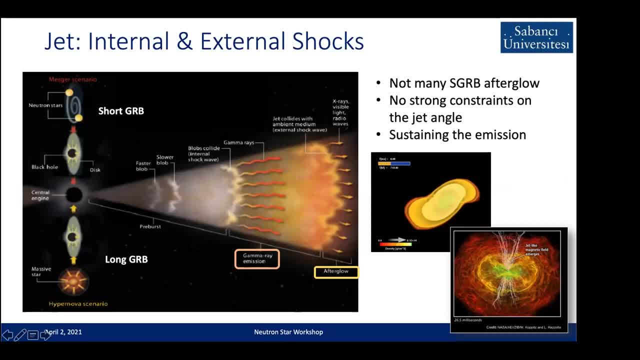 And I didn't. I didn't say anything about the long GRBs, How you know what is creating long GRBs, But because, remember the spectrum, energy spectrum- it's pretty consistent, It's pretty uniform in a sense. 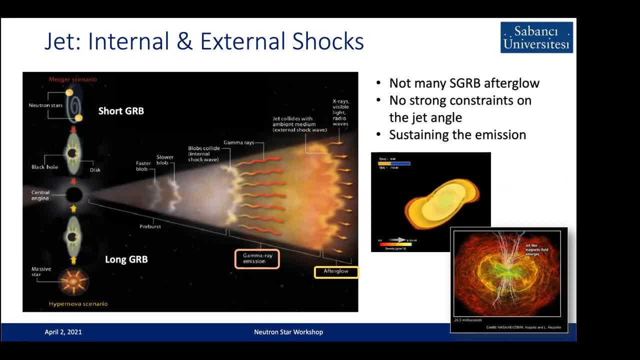 You know, it doesn't matter what duration it is. We think that emission mechanism has to be similar for short and long GRBs. Whatever the you know the progenitor may be Okay. So the emission mechanism, one of the most popular view is that the- you know the GRB has to be in jet, somehow in collimation, to account for the energy that we see. 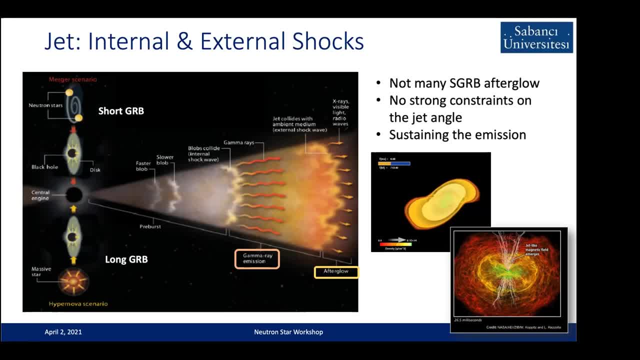 If it's, you know, if you see this much of energy, And then if it's emitted isotropically, then the estimated energy, the emitted energy, is actually huge. It's like too much So so we can't really explain. 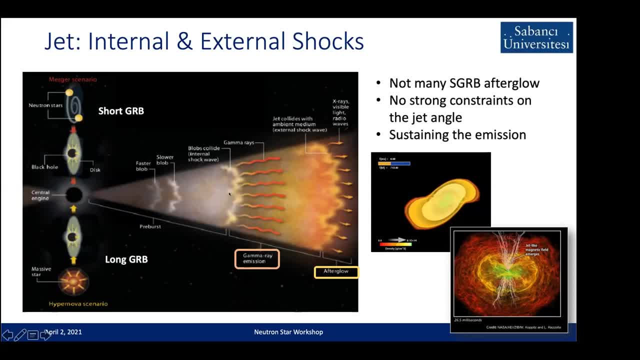 So we have to have a collimation? We do have some evidence for collimation also: the jet angles from the long GRBs. So in within the jet there's some sort of ejecta that has like a slower and faster speed. 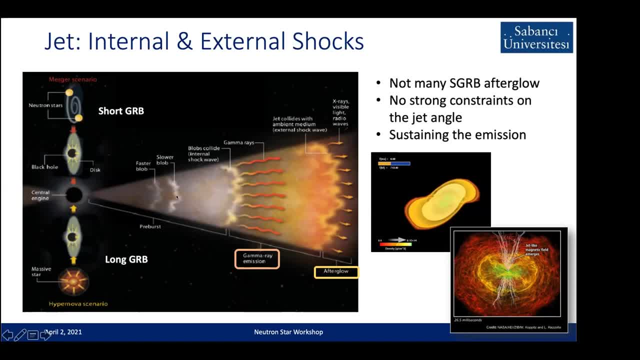 And because of the difference in speed, and these are all kind of relativistic, you know, speed, Because of these differences in speed they collide with each other And then somehow the magnetic field is created there And then, you know, because of the Fermi acceleration mechanism, within that those colliding shells, the electrons, the seed electrons, within that shell gets, how do you say, gets accelerated. 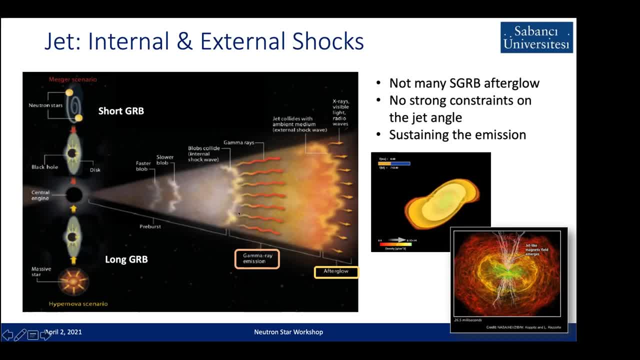 And radiates And that's what we see as gamma rays And that's why we see the non-thermal radiation, non-thermal spectrum. And then after that, this shell keeps expanding and expanding and encounters interstellar medium, And that, when the jet collides with the interstellar medium of less density, then that's what creates X-ray, visible radio as an afterglow. 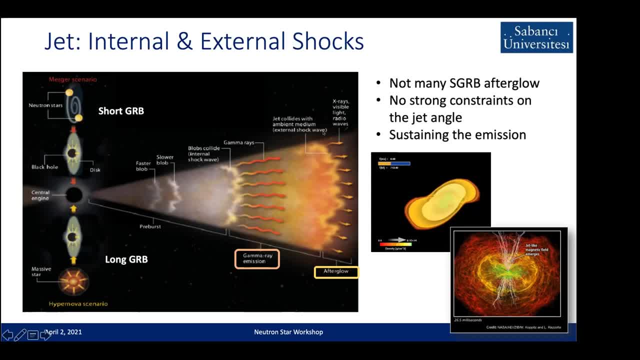 And this happens, of course, after the gamma ray burst And also happens in lower energy, Because the ejecta is already, you know, slower And short GRBs. yes, it's. the most popular theory is the merger of two compact objects, two neutron stars maybe, and colliding into black hole. 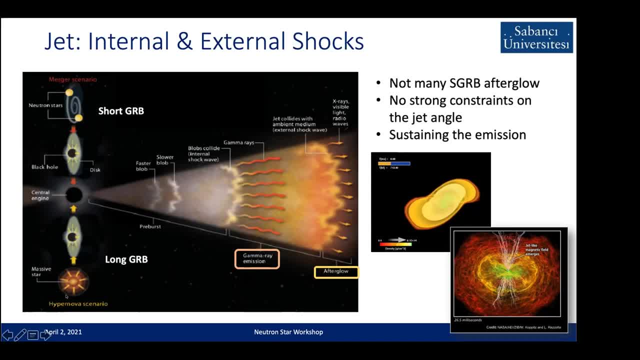 The other, the long GRB scenario Is: yeah, some people call it the hypernova scenario, But it's a massive star. It's a core collapse of a massive star. So the massive star, you know, collapses into, on itself. 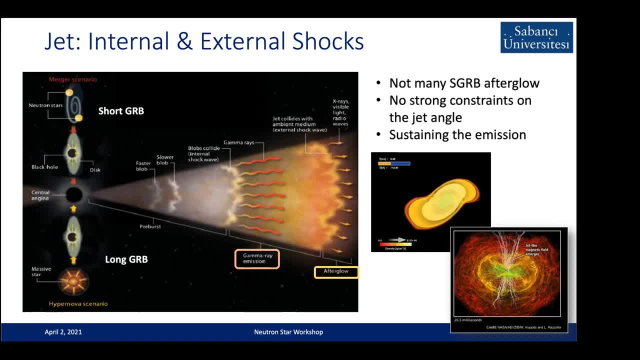 And then it explodes And then it turns into a black hole, Okay. So the problem with the short GRBs of few seconds that we observe is that few seconds is too long for neutron star merger, Okay, And too short for a long GRB. hypernova scenario, the collapse star scenario. 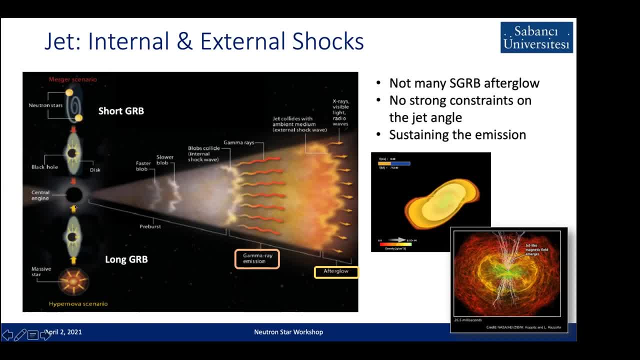 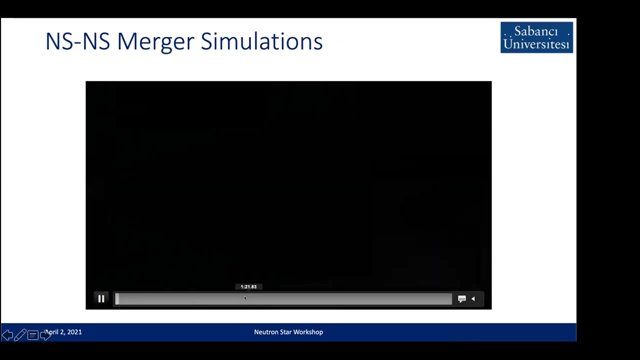 So that's why, you know, people are trying to get more information and try to refine the theory so that we can explain what we observe, And here's a simulation. actually, I have a video, I don't know if it's going to show. 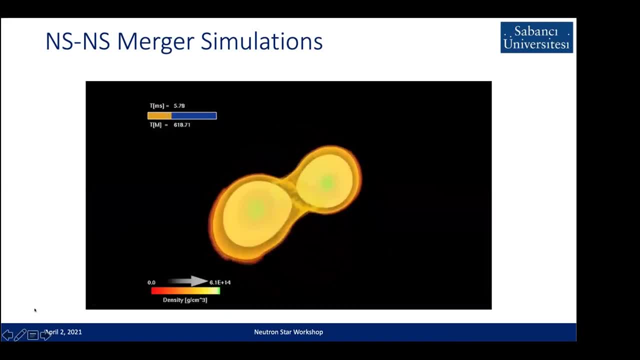 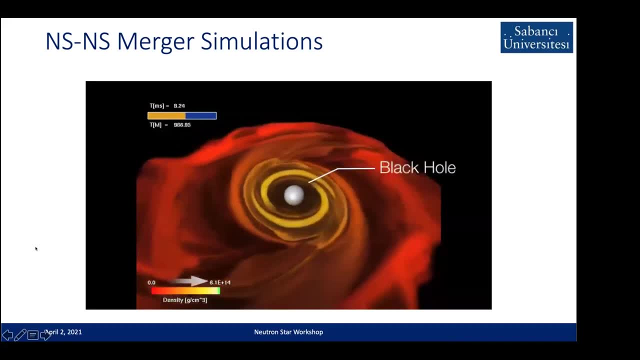 Can you see the video? Yeah, Yes, no problem, All right, good, So you can see these two stars kind of merging with each other, And then black hole is formed in the middle, And again, this is in milliseconds, tens of milliseconds scale. 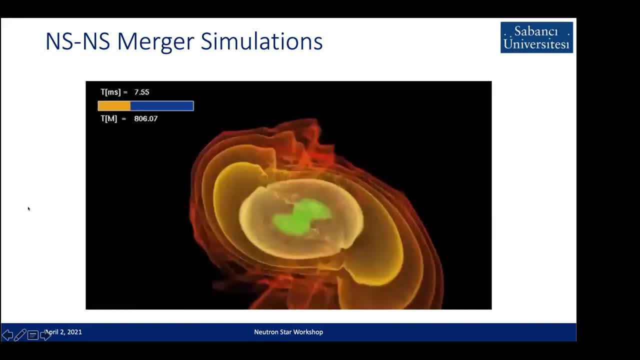 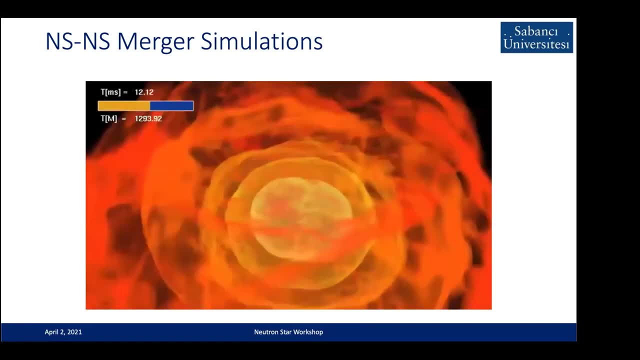 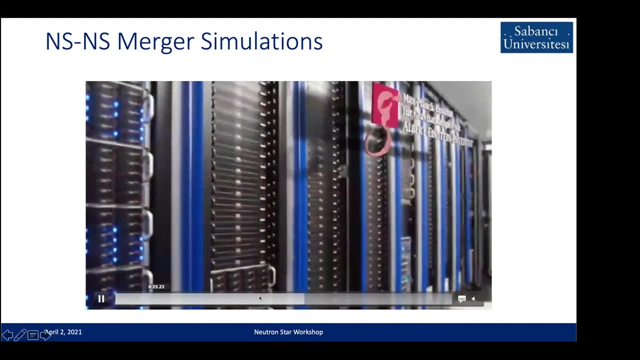 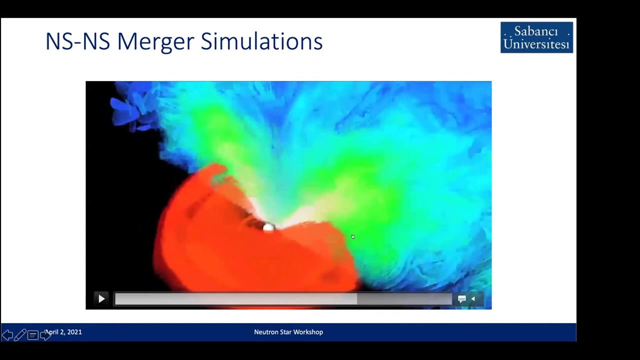 And then it forms some sort of accretion disk around the black hole. But apparently this black hole, the accretion onto black hole, only happens, you know, dissipates in like a few tens of milliseconds, I think most. So that's why, you know, it's really hard to sustain the emission for a few seconds. 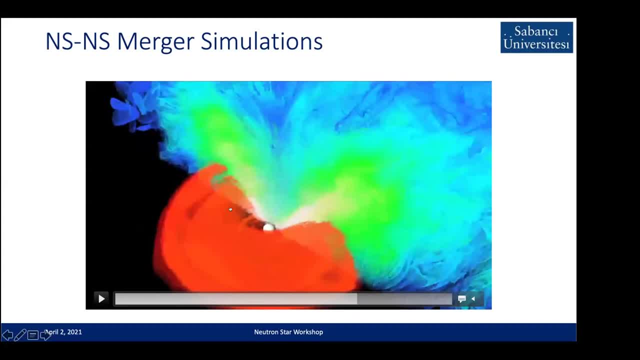 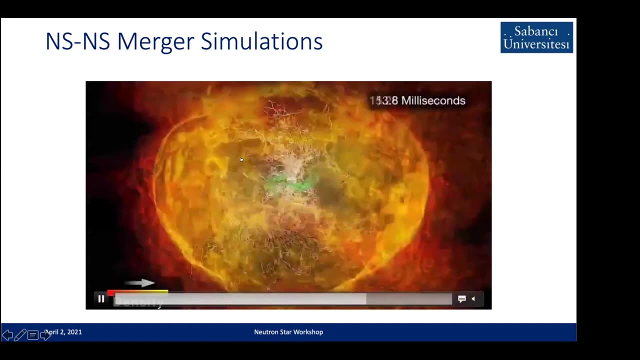 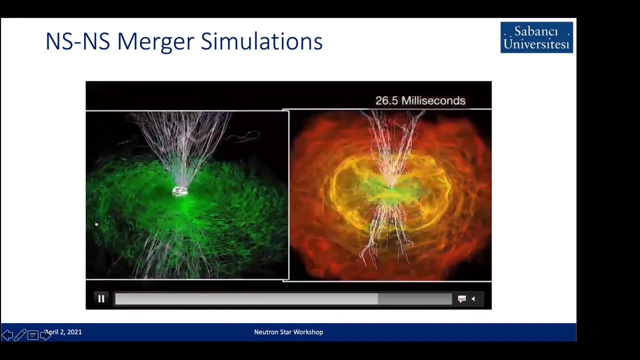 And then on top of it, this simulation also shows that this is the matter: density that you see. So the blue and green are the magnetic field actually, And you can see that these lines, you know it kind of entangles And then it finds some sort of in again, like 26 milliseconds or so. 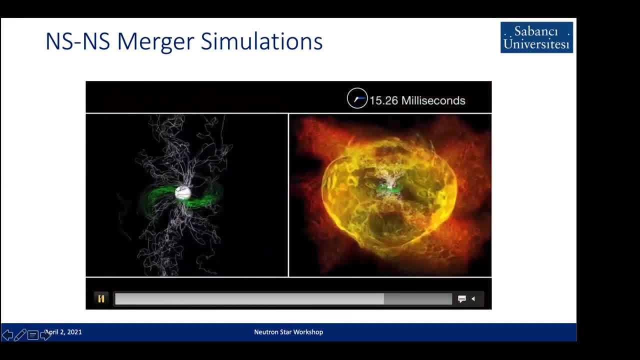 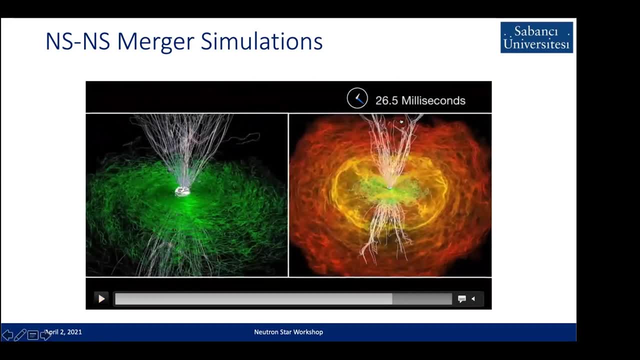 It comes into like a jet shape. There you go. So in 26 milliseconds It made the magnetic field line became some sort of jet shape And this may be, you know, driving the gamma, making the gamma reverse along with this electromagnetic field line. 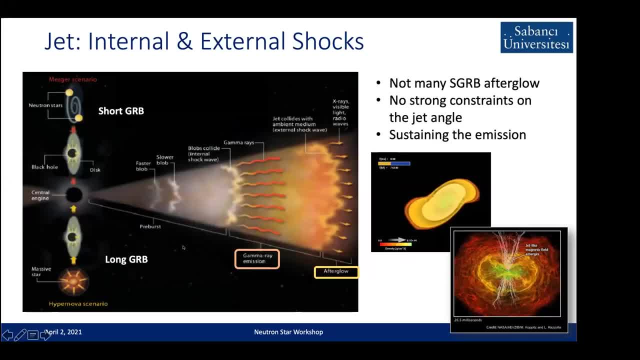 And that is great because, yeah, so here the collapse happens And however it happens, it happens, And then the central engine is ejecting this, ejecta, Fine, But how to launch these jets is another challenge, And you know, for both scenarios, because it's like so much dense. you know environment. 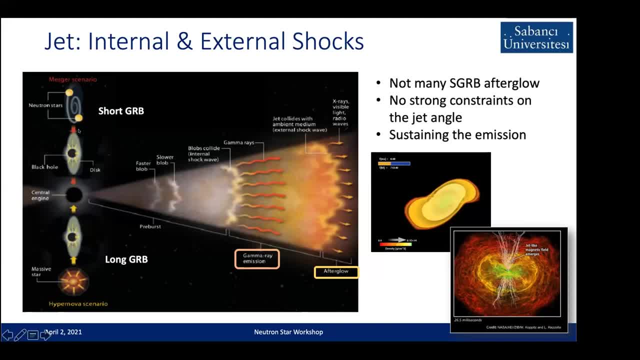 And also, you know, in the black hole, the neutron star merger scenario, you have to kind of sustain that central engine, Okay, So one of the scenarios that they're suggesting is that this forms a magnetic field And then, like those, magnetic field can somehow sustain that radiation. 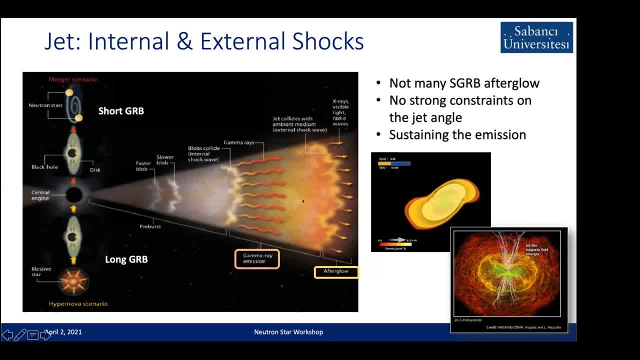 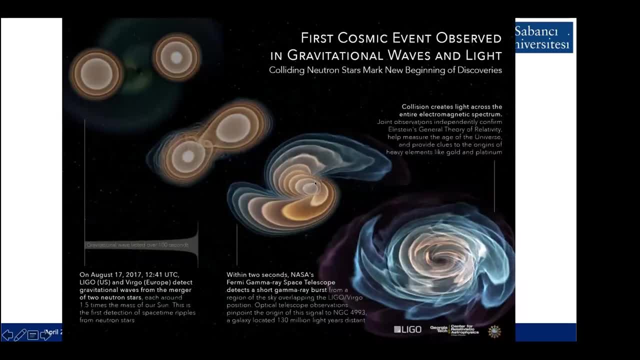 And CNEM. I think it's going to talk about that a little bit, Not necessarily for short GRBs, but in general about afterglow and magnetar, And very recently, 2017, in August- you all have heard about this, most likely. 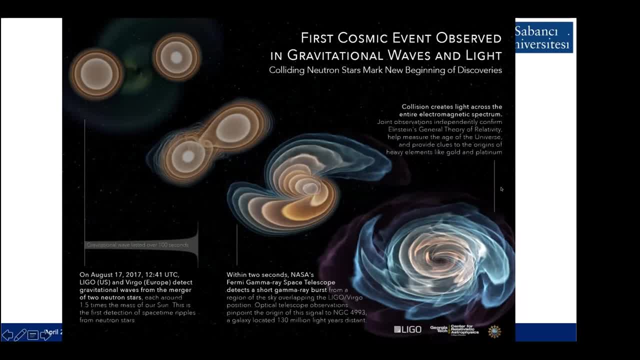 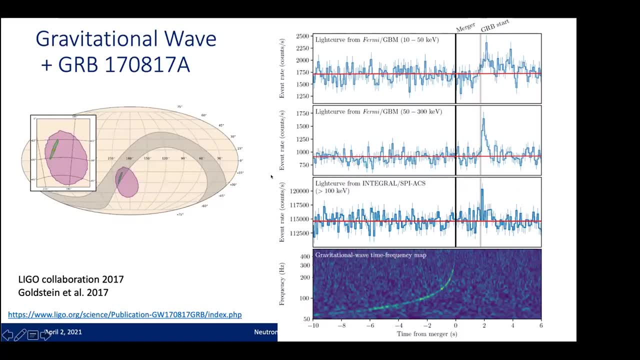 Right LIGO detector detected the gravitational wave from neutron star merger And along with this, a GRB was detected. It wasn't triggered. It didn't trigger the detector, But afterwards, when they searched after this gravitational detection wave detection, they found in GBM and then also integral speed have observed this event. 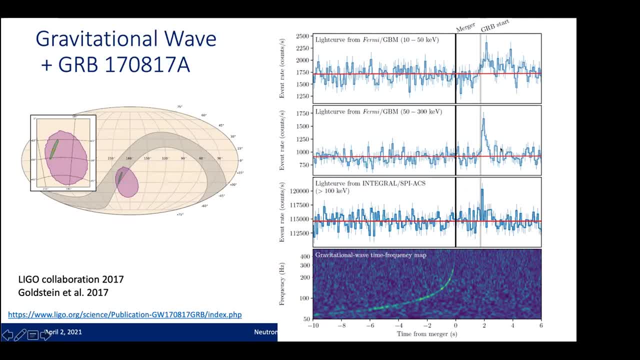 It's very, very faint. It's much fainter than regular short GRBs, But they did find this And there was a two-second delay. So from here you can. they were trying to estimate the propagation time of the gravitational wave and light propagation speed from this delay. 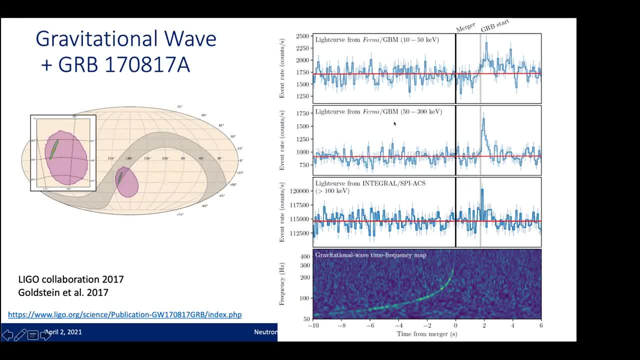 Like I said, GBM does not have a very good location capability. So, you know, when you see a burst like this, you know we're not sure if this is from. you know exactly that location of this merger or not. 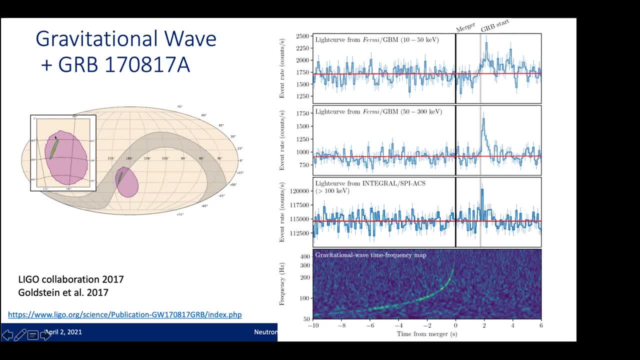 But from here you can see that error circle of this is LIGO error circle and this is GBM error circle And these gray lines are speed bands, You can say observational bands, So you can see that all of them coincide at the location of this LIGO event. 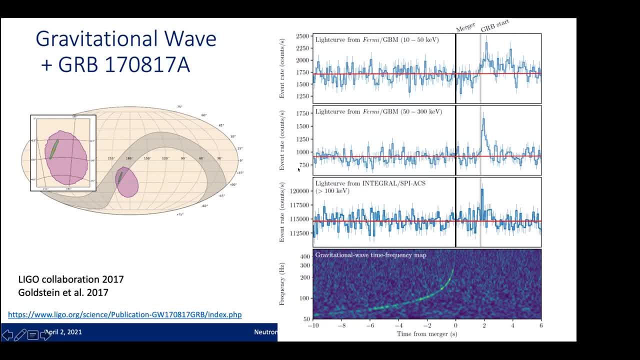 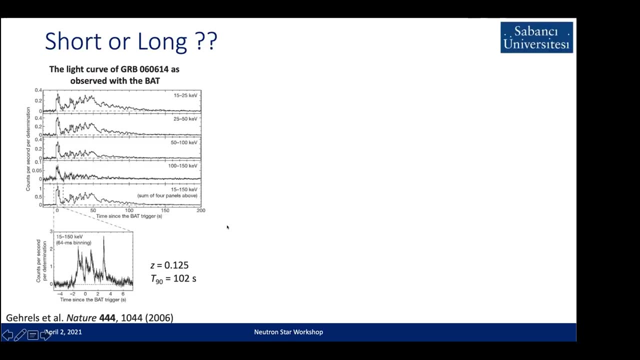 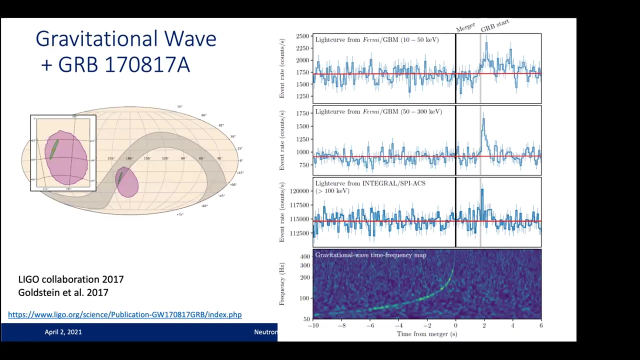 So this is. I think it is pretty convincing. So we did see a first kind of evidence of short gamma ray burst associated with neutron star merger. So that's a good thing. So that's like a first direct, Direct evidence that we observed. 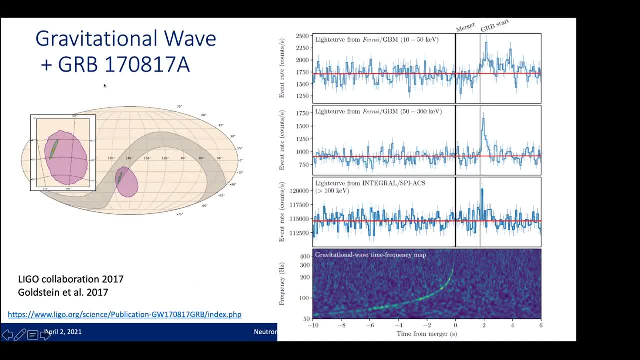 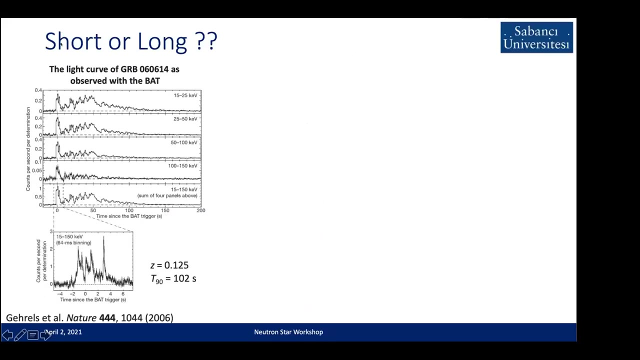 And there are a lot of effort trying to detect another one and also try to do offline search trying to detect, find similar short GRBs, that is like less energetic, like this, and trying to match the gravitational wave data. And, as I mentioned, there's a short GRBs with some extended emissions or maybe it's a long GRBs. 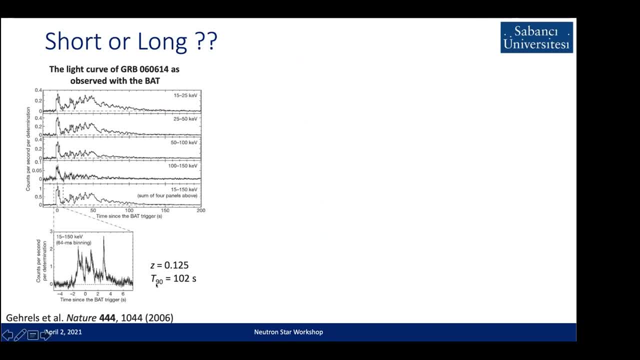 We don't know. So this one in 2006, this was observed And this was kind of first case that we observed something really, really puzzling. So this was observed with bat, swift bat, And the duration, As you can see from the light curve. 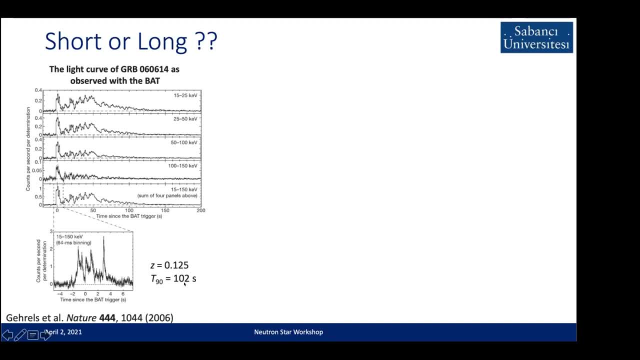 The duration of this event, Determined with bat, was 100 seconds. So of course it's a long events, right, Just going with the duration. But for long events- And this happened pretty close- Z is 0.1.. 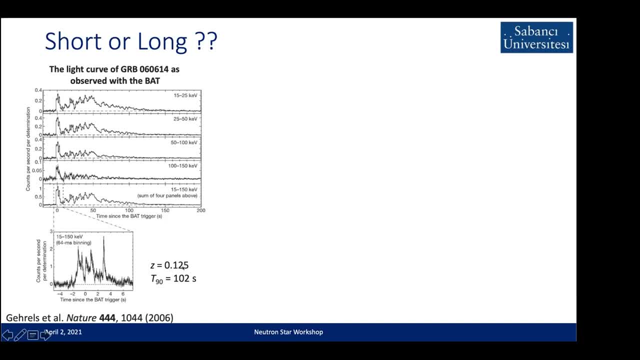 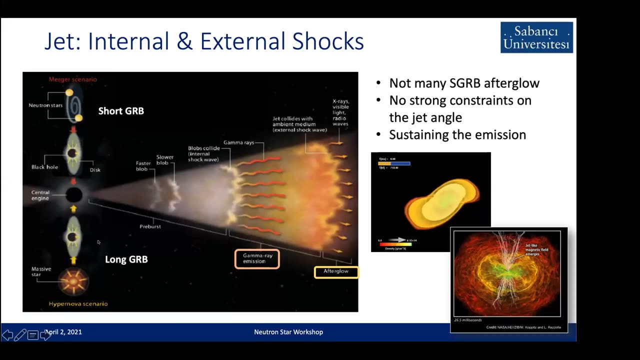 So it's a, you know, by GRB scale, it's a pretty close event. And if the event is this close and if this event is long GRBs- and then it was caused by, you know, this massive star collapse, Then there has to be a supernova signature that's visible. 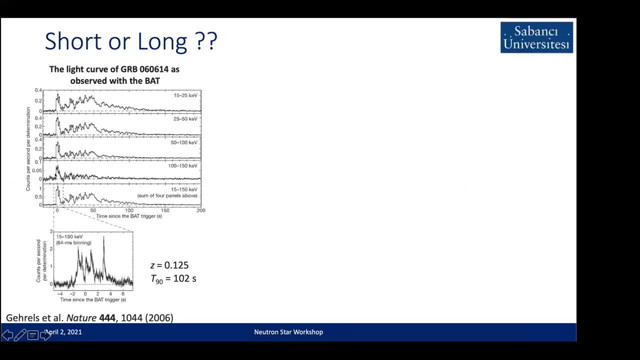 In optical band. So there was extensive search for supernova signature and they did not find anything. So they were really puzzled, Okay. so this looks like a long event, But you know we don't see any. you know supernova signature. 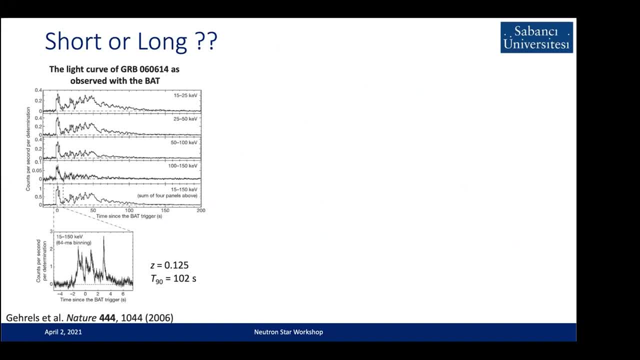 Which should be visible at this close distance, And on top of it there are some other spectral log information that we got from here From this event wasn't matching the long GRB property, The characteristic that we have seen before, And also, if this was observed, this would have been observed with the Batsy. 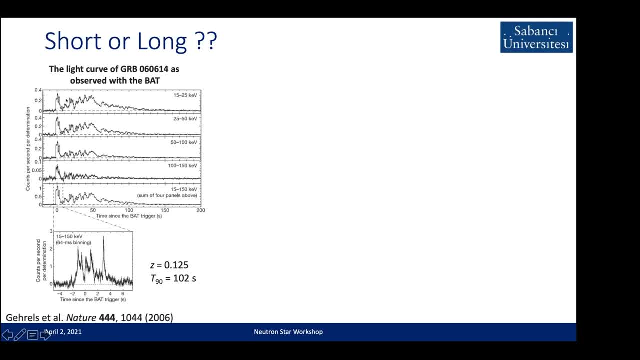 We did some simulation And we saw that in Batsy This faint Tail emission- Extended emission- wasn't observed, So the Batsy would have classified this as a short event. So there are cases like this And recently we have two more cases. 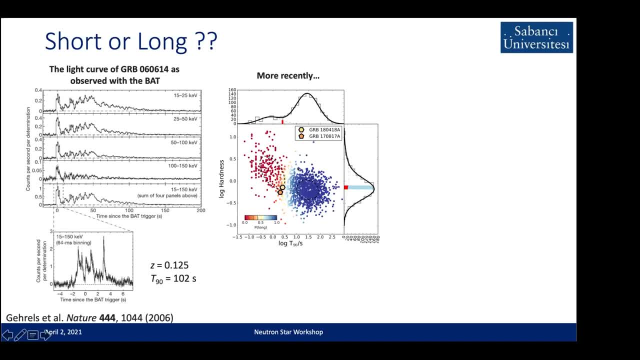 That's not just from the duration, But overall property of afterglow hardness, like everything. When we compare it, When we look at it, It's not really matching a short GRB, Or it's kind of somewhere between short GRBs and long GRBs. 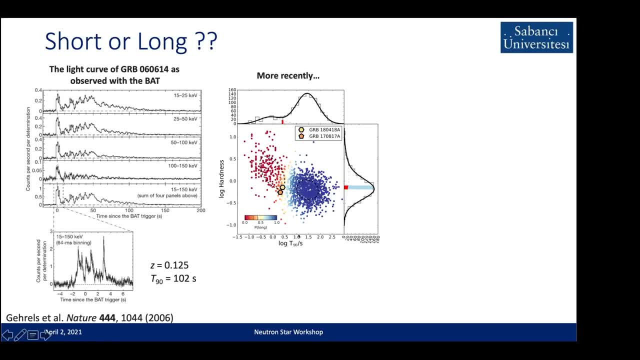 So you can see, this is again the hardness ratio And duration information And these two events are fitting right in the middle. So it's not clear. And also we have searched something similar to these events: Short GRBs with extended emission Using Batsy GBM and Swift GRB data. 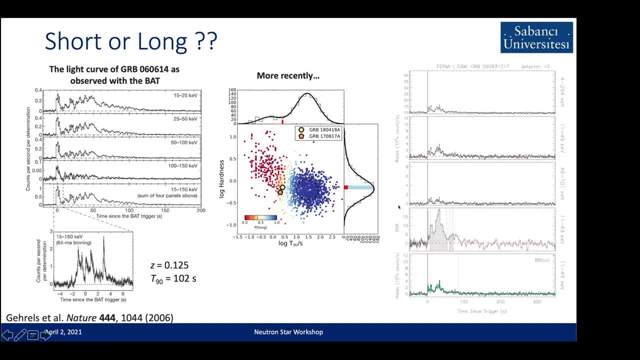 And we have found about 30, 50 probably, total events That has. you know, this is the one that we found. It has a very, very short spike But it has kind of hump emission, afterwards Extended emission. that's much dimmer. 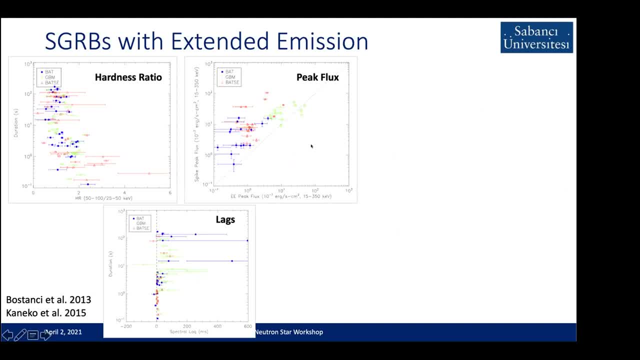 But still this is bright for our detector. And then when we look at these extended emission versus the spike, We see that yes, we still see hardness ratio Differences- Not exactly differences, But you can see the tendency again That short, this is duration here in hardness. 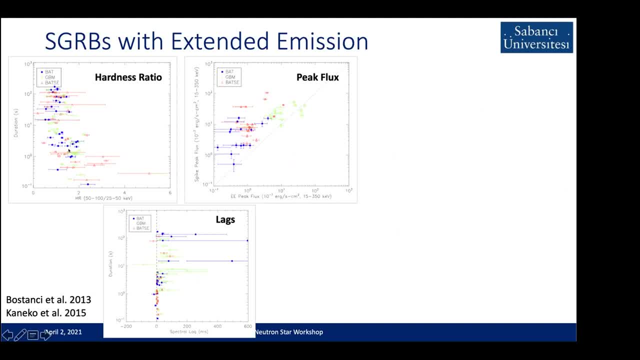 Short spikes right here have a little bit harder spectra compared to extended emission part And peak flux. Actually there's a little bit of positive correlation between the extended emission peak flux and spike peak flux. So when the peak flux is higher in spike, extended emission tend to be brighter. 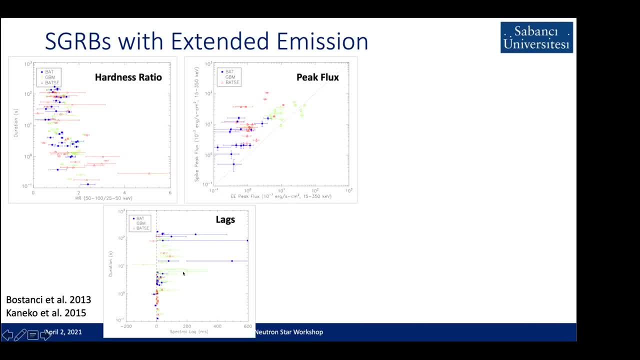 But again, it's not very strong correlation, But we can see the relation. And then also, when we look at the spectra lags, we can see that. So this is spectra lag. So this means the higher energy component comes a little bit before the lower energy component. 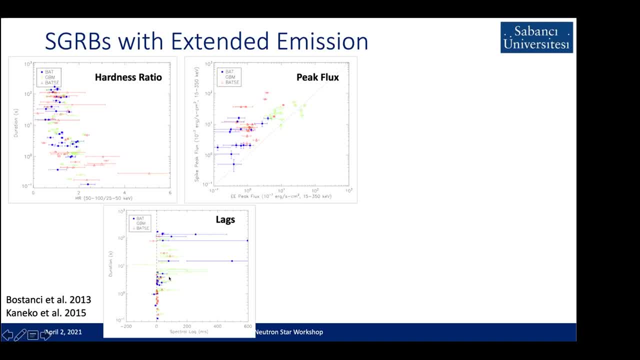 And we can see that extended emission. the lags are a little bit more And lags are usually observed for longer GRBs, long GRBs, So this is a little bit more like a long GRB. Long GRB properties characteristics. 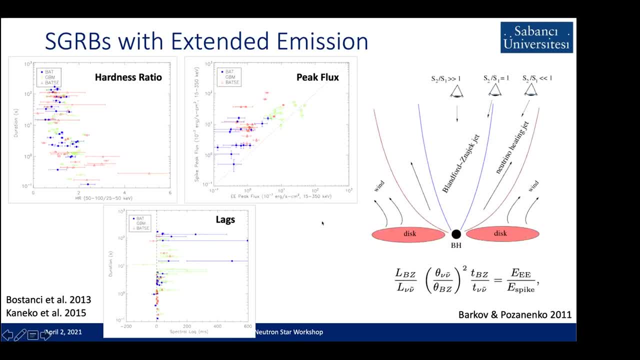 And what could explain this short burst and extended emission, the difference between them? This is one model by Barkov and Potanenko in 2011.. And they're suggesting two component model like this. So you have a black hole with disk. 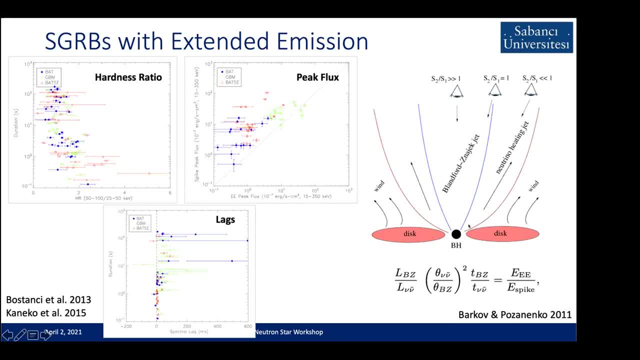 And first neutrino heating happens From this merger. there has to be neutrino and anti-neutrino And they have to make pairs. So those pair creation actually is what we see first as the short spike And then afterwards this electromagnetic Blanford generic jet is what we see as extended emission. 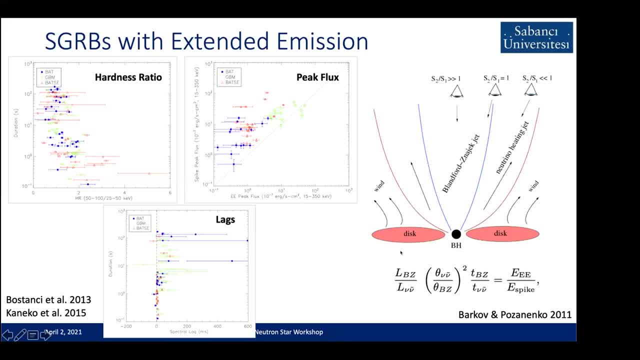 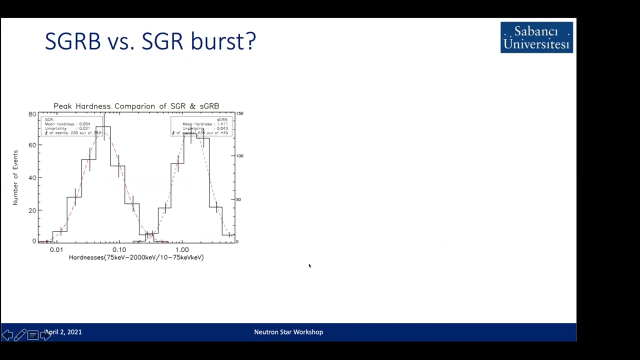 That's their suggestion And we did test using this And we tried to constrain this ratio of opening angles And we see that for all cases that neutrino jet is wider than Blanford generic jet, this electromagnetic jet, And finally- yes, this is my last slide- 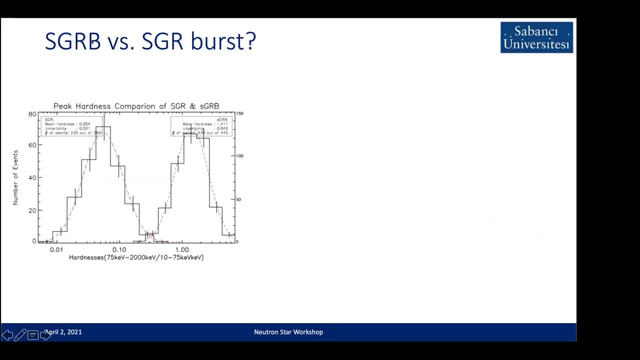 Finally, so I want to mention SGRs, because you know the earlier talks. they talked about magnetars, GRB, short bursts from magnetars. So when we observe a gamma-ray burst, short gamma-ray burst, how can you tell that it's not the SGR but it's short GRBs? 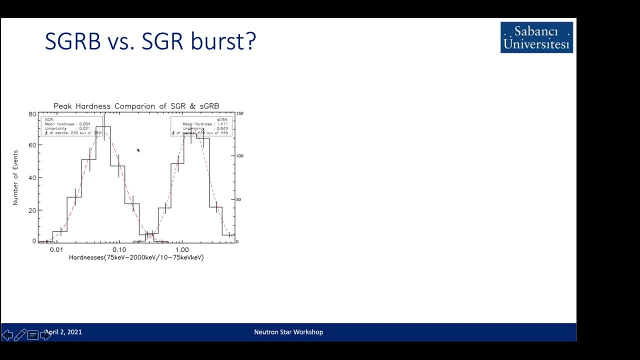 The most clearest difference is the hardness. Soft gamma repeats. Soft gamma repeaters are soft gamma repeaters And it's repeaters, So it comes from the same place And short GRBs never repeat So far, never repeated So soft gamma repeaters. hardness: you can see quite distinctively that this is much softer. 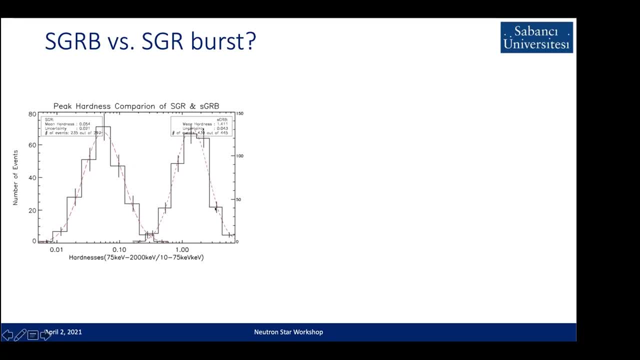 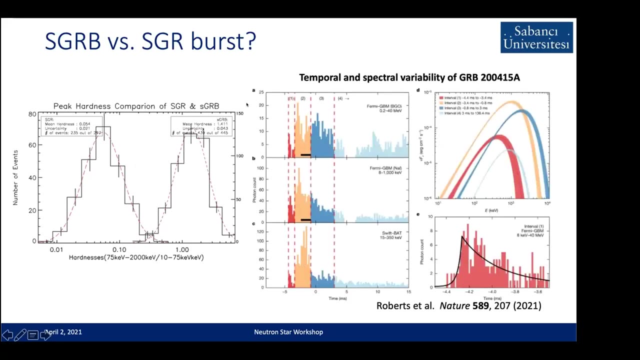 This is short GRB. The GRBs are harder, much harder. So from here spectral characteristics. you can see, And for SGRs Spectra are usually thermal or two or three thermal components model, But GRB spectra is really non-thermal. 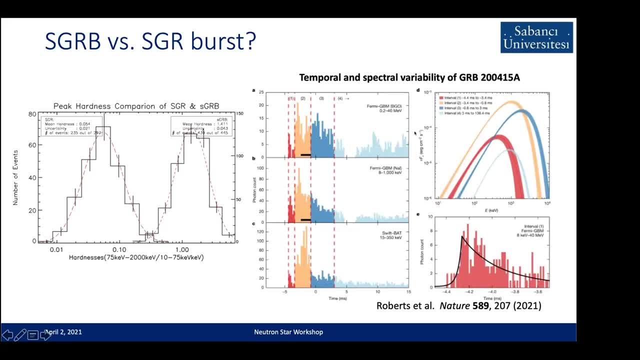 And lastly, I'd like to mention this one. So this is. this was just published recently. This event was originally classified as short events And you can see the millisecond here, the time scale, The event itself is very, very short. 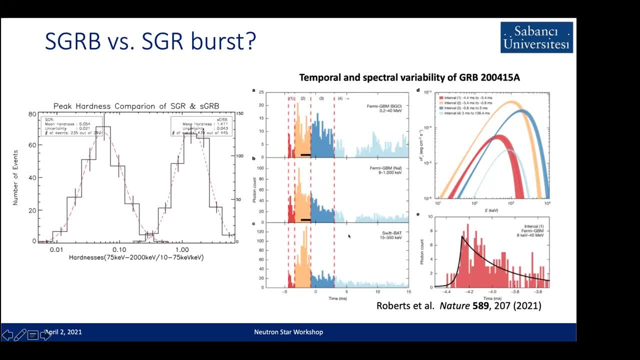 But it's pretty variable And, in addition, the spectral characteristics Spectra was pretty, it's very hard actually And it's a little bit different from what we see or what we expect from short GRBs, But it was very similar to the giant flare SGR giant flare spectral characteristics that we have seen before.